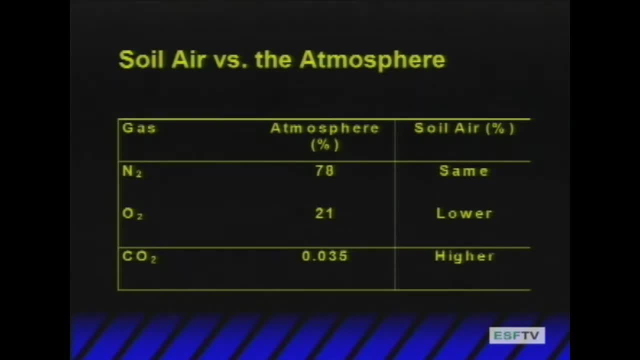 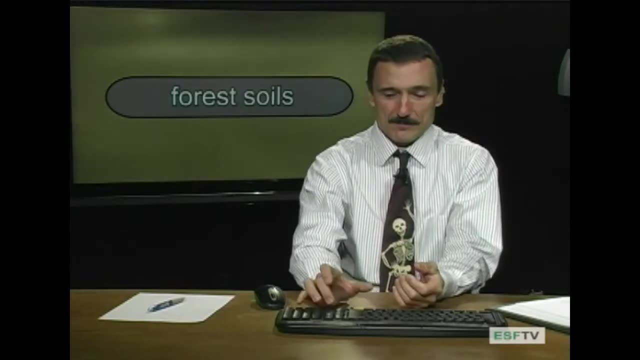 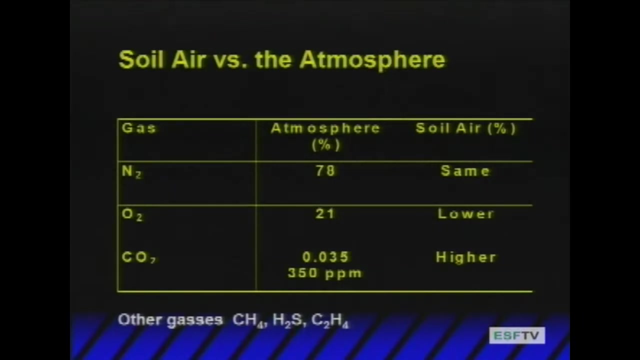 And the question becomes how much lower or how much higher? And the answer really really depends on soil physical properties and soil biology, And so we'll explore that today. Some of the other gases, methane, hydrogen sulfide, some of these other very small concentrations, they're important. 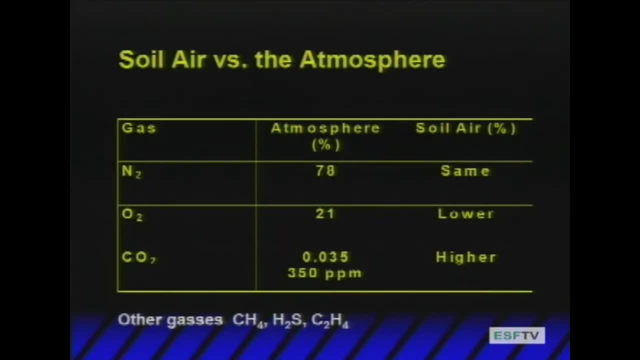 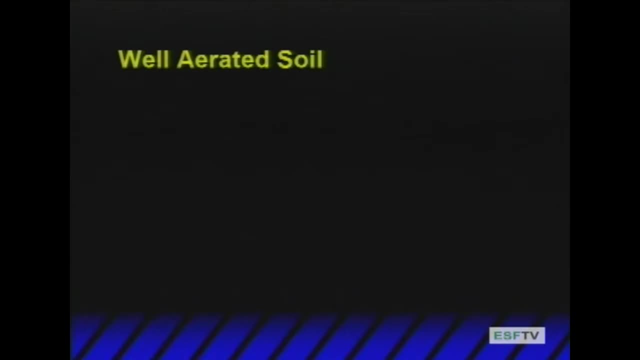 greenhouse gases, But again, today our focus really is on those that really apply to plants, and we'll be focusing mostly on oxygen and carbon dioxide. So what is a well-aerated soil, you might ask, And I may ask you on the next exam And if we 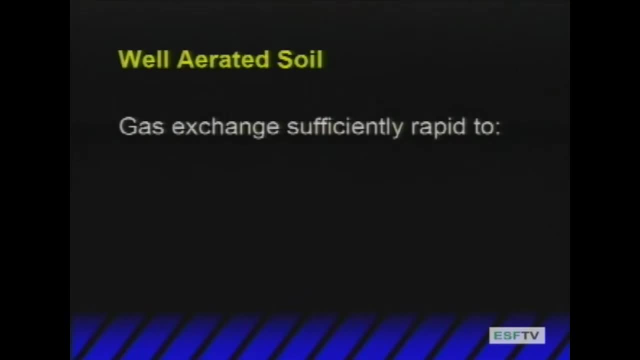 would define a well-aerated soil. we would talk about a soil where the gas exchange is sufficiently rapid. There's a certain amount, those four-to-five-year-olds- there's a certain amount of fluxes, that flux of gas that we talked about earlier, that arrow going from the soil to the 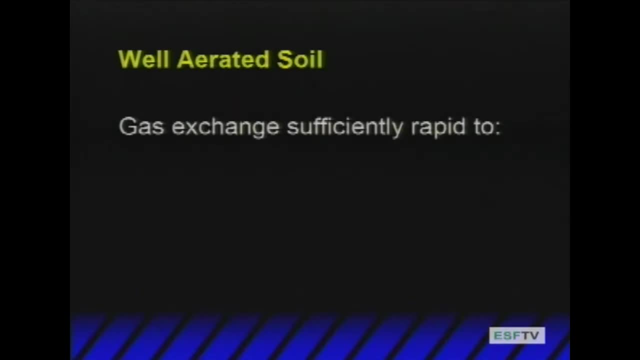 atmosphere that has to be sufficiently large so that certain things happen, And one, an important part of that is that the oxygen in the soil is replenished And at the same time that oxygen is used up, and while that's being used up, carbon dioxide is built up. A lot of respiration, a lot. 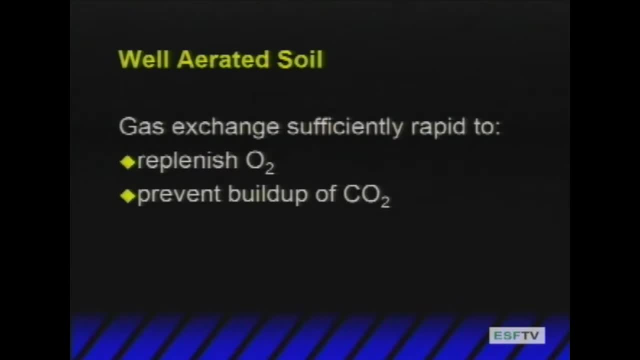 of activities. the roots, all of the biota are producing carbon dioxide And if that was allowed to build up to great levels, then that's a lot of oxygen And if that was allowed to build up to great levels that kind of reduces the biota, their ability to function. In the same way, if oxygen gets too low, 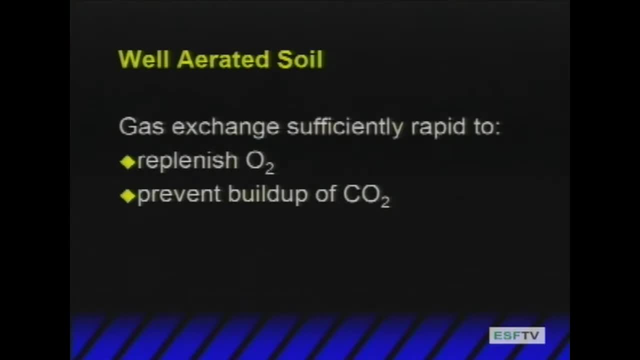 the respiration doesn't occur. So a well-aerated soil is one where this process of gas exchange allows sufficient exchange of oxygen and CO2 to prevent this buildup of CO2 and to encourage the continual replenishment of oxygen. So that's a well-aerated soil. very succinct definition. 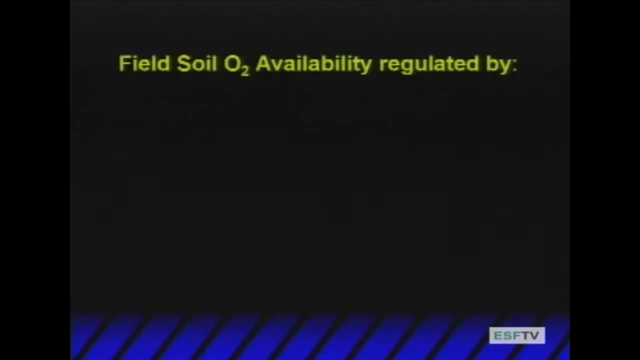 And what about this oxygen in the field? So, if we look at soils, what controls the availability, what controls the concentrations of oxygen in the soil? And there are a few properties that we can talk about and think about, And the first, the most obvious one, soil macroporosity. 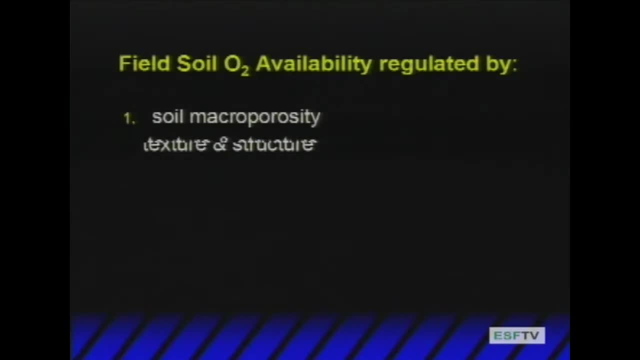 And so in macroporosity we have some generalities we made about texture and structure And we had sandy soils tend to be very high in terms of macropore space compared to clay soils, And we had some structure: well-structured soils versus poorly structured. So essentially those large pipes that allow for macropores. 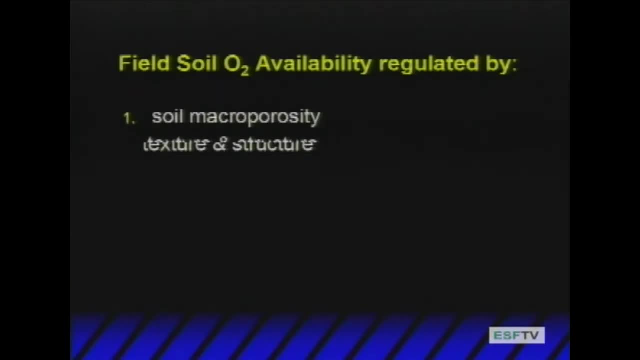 these large spaces that don't hold water against gravity. this is where these exchange take place, So soil macroporosity is very important. I don't know if you, my slide is kind of interesting. I hope yours reads the same. It looks like a Cyrillic texture and structure. 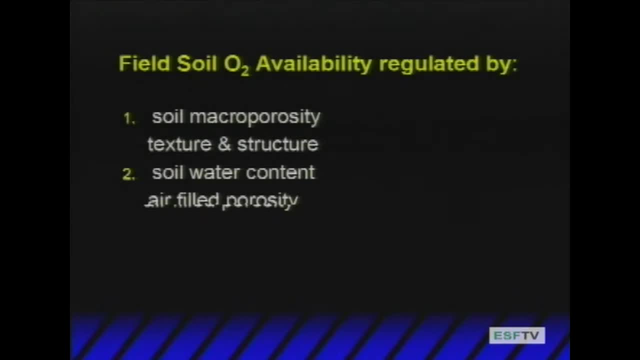 Ah, it just came back, Okay. the second part of that is water content. So, remember, we have these pores: 50%, ideally, would be filled with air, 50% with water. So if all of these are filled with water, 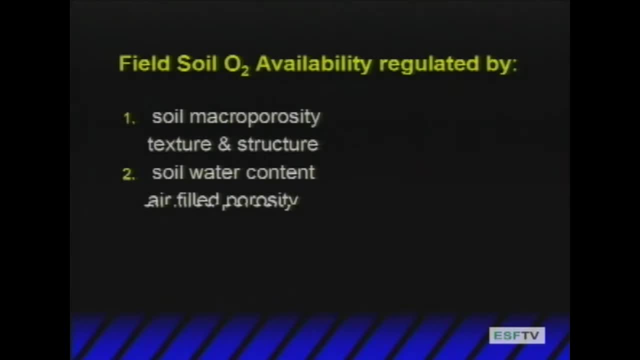 the air-filled porosity is going to be low. The exchange is very slow. The exchange in air-filled pores is about 10,000 times more than the exchange of oxygen in a water-filled pore, So soil water content has a direct impact on this process. 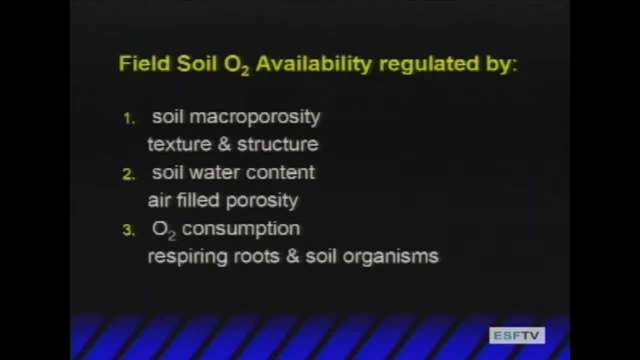 And finally, the rate of consumption. So we have plants, we have biota, we have a variety of these organisms that are aerobic, They are consuming oxygen and their rate of consumption draws this down. So the greater the rate of consumption. 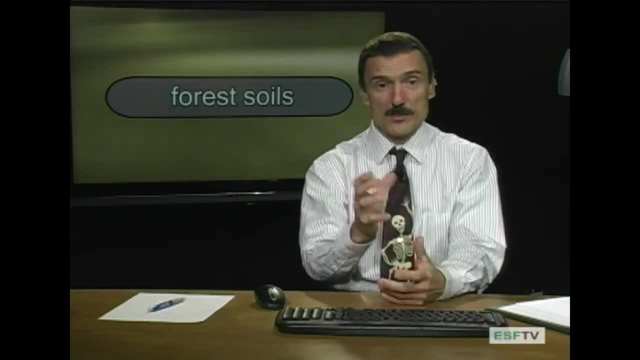 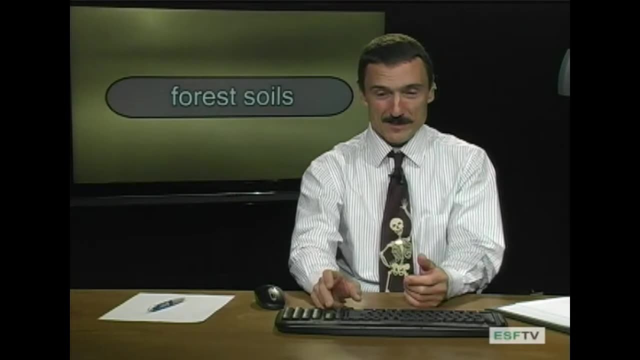 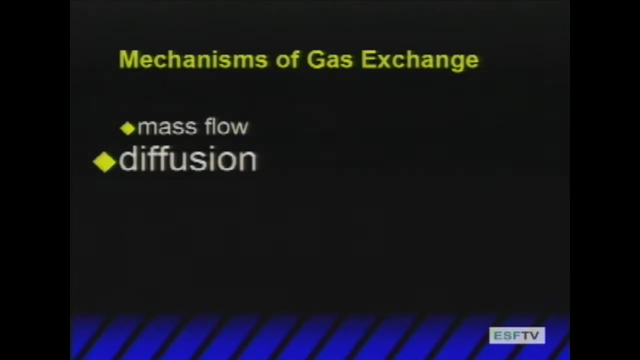 okay, the greater the need to have this process occur, this exchange of oxygen allowed from the atmosphere into the soil. And who could forget the soil organisms? So what's the mechanism? There are two possibilities. right, There's mass flow, just the mass flow of air movement. 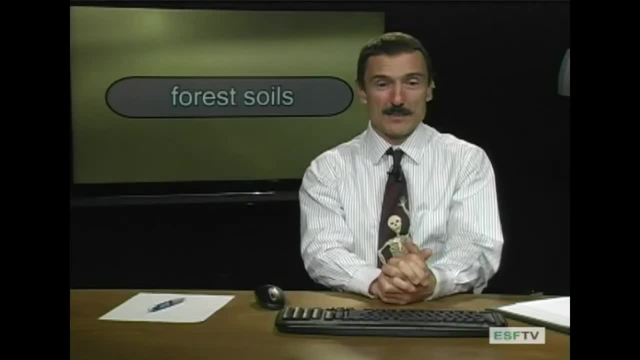 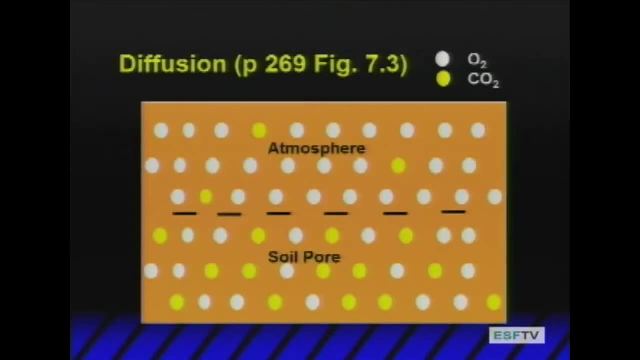 and there's diffusion And of course by this slide it kind of implies that the real important mechanism here is diffusion. So what is diffusion? Okay, diffusion is the movement of gases to establish an equilibrium against a gradient. So this slide here depicts the process. We have the white gas in the atmosphere. the whites represent oxygen molecules. 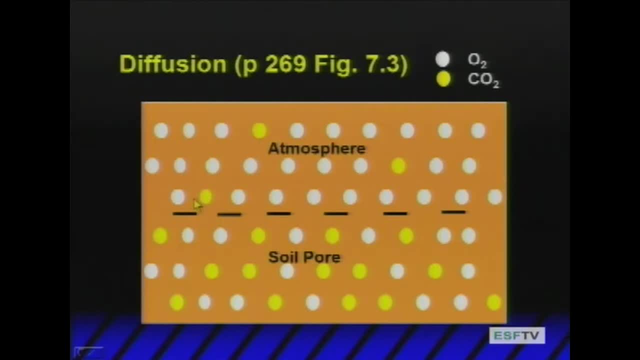 and we have the yellows representing CO2.. So where is the gradient? So in the atmosphere, the concentration of O2 is much higher than the soils, and the reverse is true of CO2.. We look at CO2 and the concentrations, the partial pressure of CO2,. 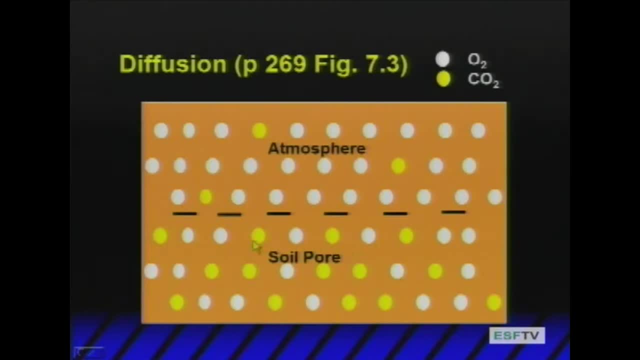 much higher in the soil. So this is a gradient and so diffusion is the movement of these gases in response to a gradient, in an attempt to establish an equilibrium. So, the carbon dioxide being higher concentration in the soil, it's being produced by a number of roots and organisms by respiration. 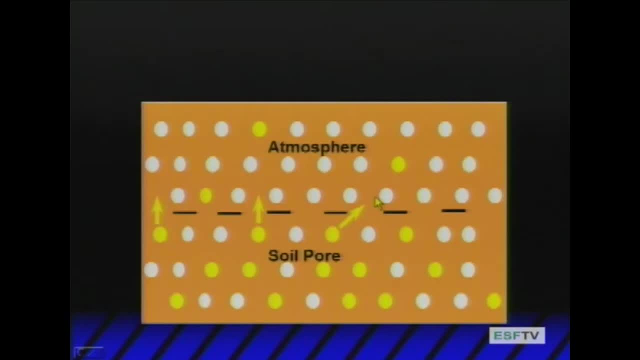 That tends to diffuse outward into the atmosphere, And the reverse is true for oxygen. Oxygen is higher concentration in the soil, sorry, in the atmosphere tends to move inward toward the soil. Of course, now we've got to think about the way this is occurring. 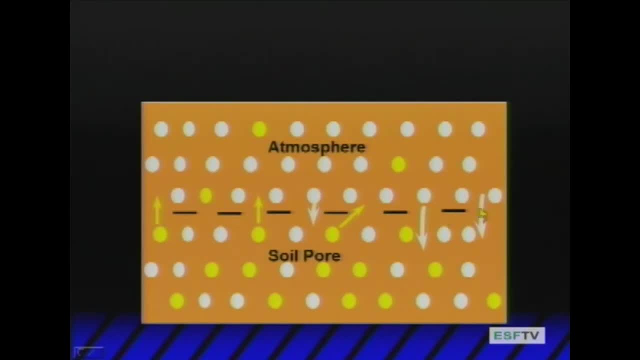 This is occurring largely through macropores, Those are those large pipes that don't hold water against gravity If they are filled. during saturation, this doesn't occur. So that in fact of soil texture and structure becomes extremely important, because it has a big factor. it's a large factor. 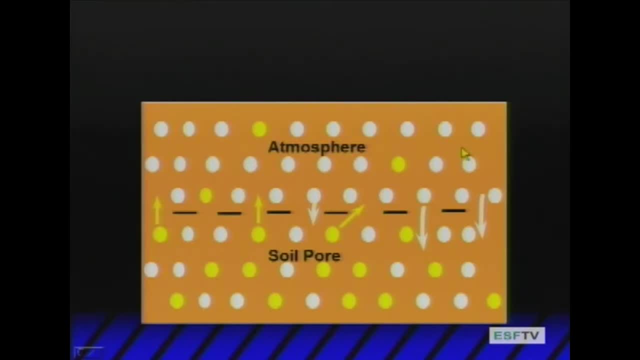 in regulating this movement, this gradient Now, that is diffusion. We look about the rates And again highlighting the importance of these air-filled pores. if you look at an air-filled pore and you compare that to a water-filled pore, the rate of diffusion is about 10,000-fold different. 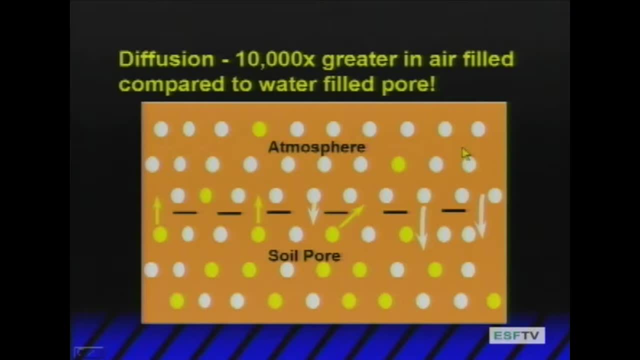 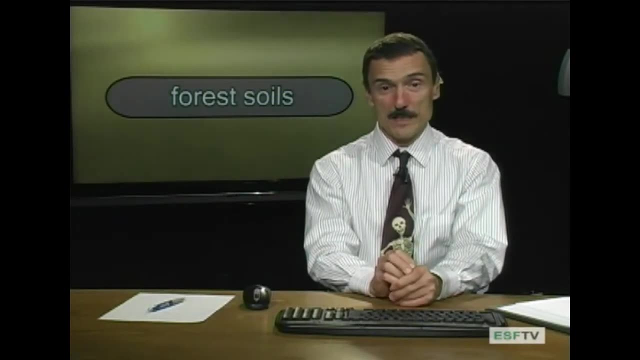 That's an order of magnitude of 4.. So you can see why we really rely on this concept of air-filled pore space. And now we kind of build on last week's work in terms of soil moisture and soil moisture retention And this directly, these ideas of diffusion. 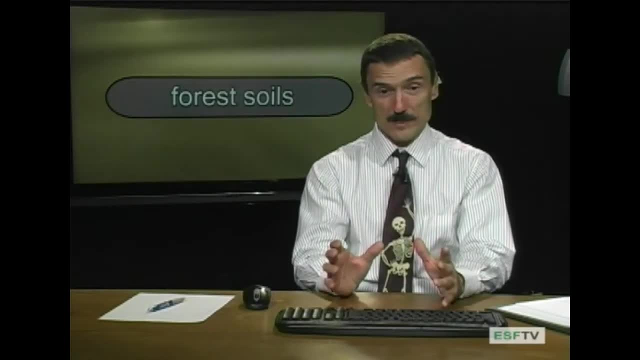 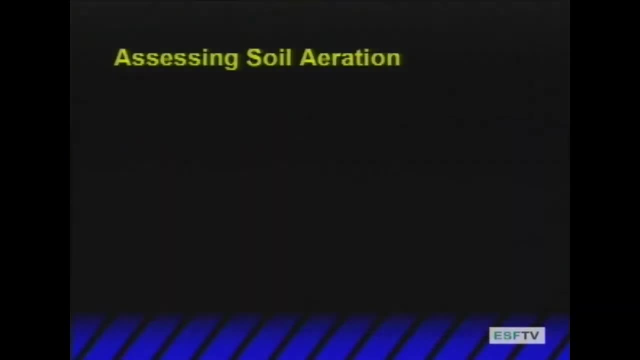 you can paste this right over our soil: moisture characteristic curves, looking for that proportion of macropore space. And we did those calculations last week in lab. How do we assess soil aeration? So we've defined it, We've kind of looked at the process. 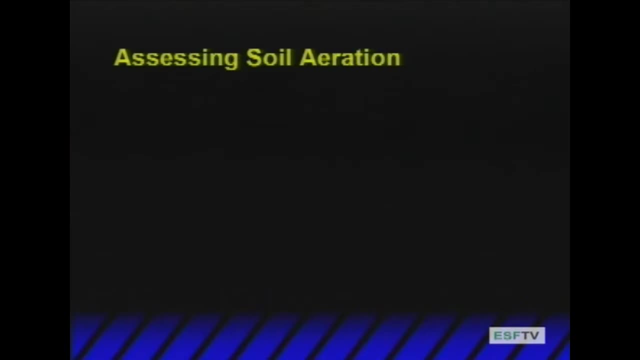 And now are there ways to assess it, quantitative ways to say, yes, we have good aeration, no, we don't have good aeration, or we have poor aeration, conversely, And so one of the, I'll give you a number of them. 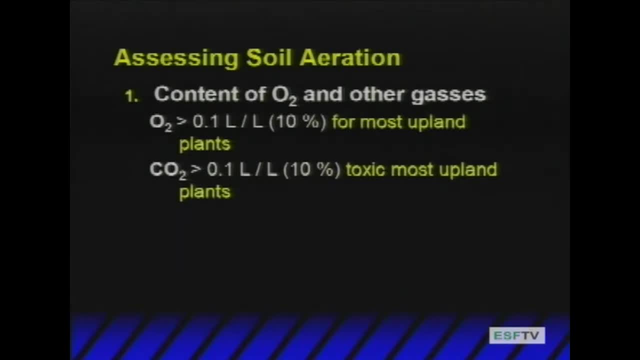 And they're just. they're no particular importance, but just in a numbered list. The first one would be obviously the content of oxygen in other gases, And just measuring the oxygen concentration in the soil would give us some idea of soil aeration. 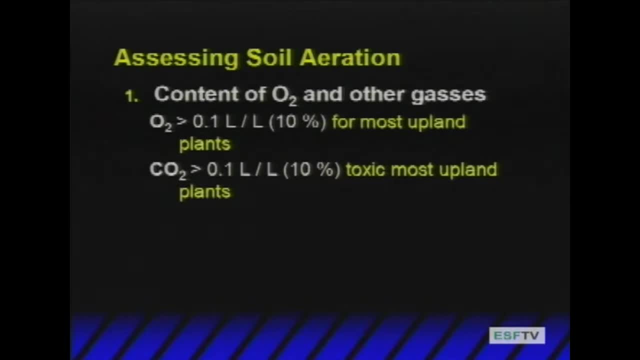 And some of those numbers. we have these rule of thumbs- and these are pretty useful to have in the back of your head, particularly during exams- is that, in general, the oxygen concentration greater than 10% for most upland pans, that's the requirement. 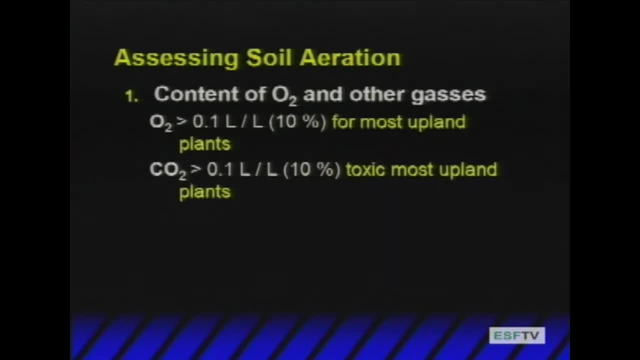 So if we can actually put a sensor in the soil and measure the oxygen percentage, the partial pressure, we say if it's 10% or above that's adequate for most upland plants. That's kind of a cutoff, a threshold, a number. 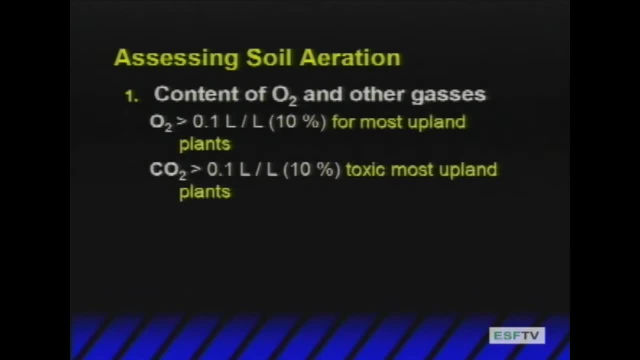 We think about good aeration. yes, let's say 10% of oxygen concentration. In the same way we can look at CO2 concentration. So when the partial pressure- the concentration of CO2, exceeds 10%, then we tend to think of that. 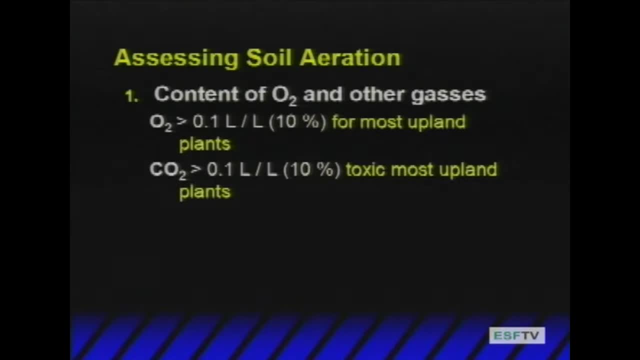 that becomes a very bad number. That becomes. that implies a toxic situation. So we could either measure the oxygen content, or we could measure the CO2 content, or we could measure the CO2 concentration and utilize that as one measure of soil aeration. okay, 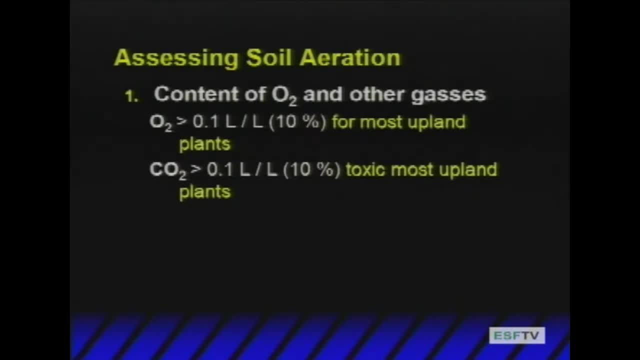 And again it's at the 10% greater, for oxygen, Plants need more than 10% and if you have more than 10% CO2, that's a negative thing. So that's a. that number is reversed in terms of oxygen and CO2.. 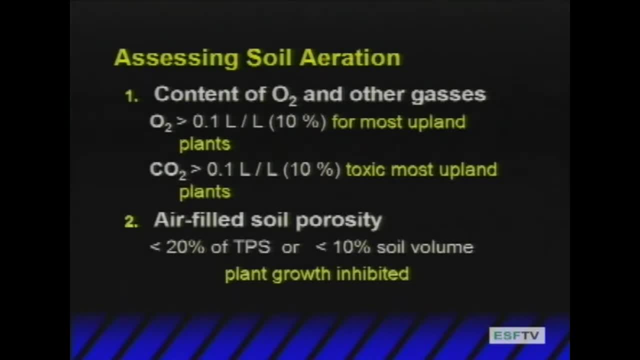 Another way we could do is just look at the air-filled porosity and we talked about the macropore space And, in general, if we have less than 20% air-filled porosity, total pore space that would or less than 10% of soil volume. okay. 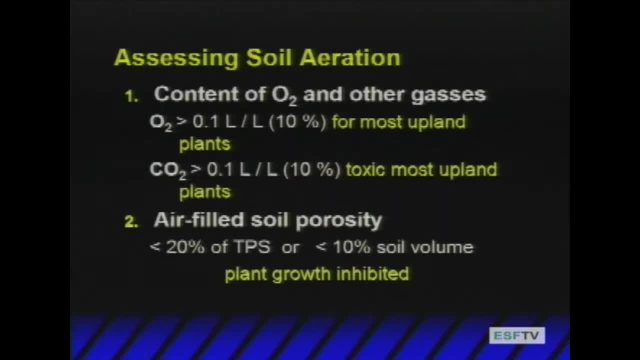 we would start to say that's kind of a cutoff. So 20% of total pore space or 10% of soil volume, that would start to inhibit plant growth. That's a fairly easy measurement to do. We could get that measurement probably right off. 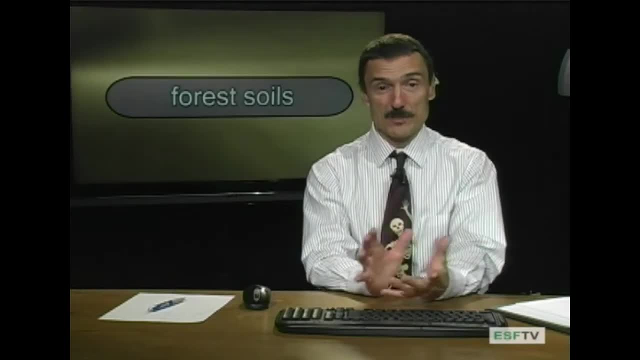 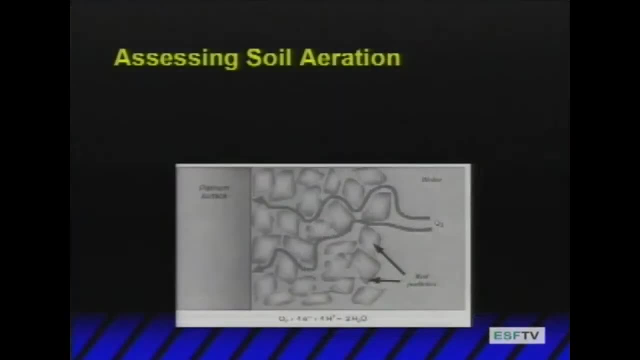 our soil moisture characteristics And we did that calculation. What's the macropore volume percentage of a soil? Okay, Here's a a little slide showing the illustration of this and showing how things diffuse. okay, and think about soil. So we might be interested in the rate of diffusion. 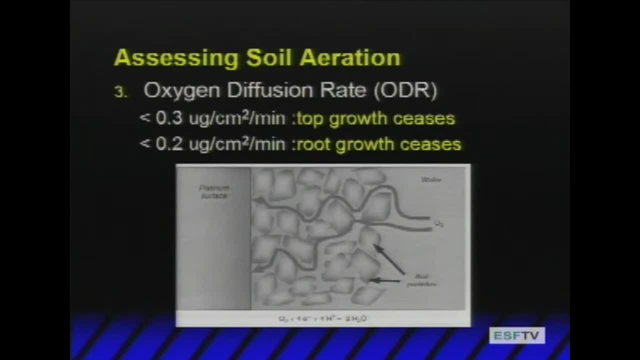 And so we could also measure the oxygen diffusing rate- That's so abbreviated as ODR, the oxygen diffusion rate, And this is a measure of the rate at which oxygen diffuses. This is actually done by platinum electrodes, and you insert these platinum electrodes in the soil. 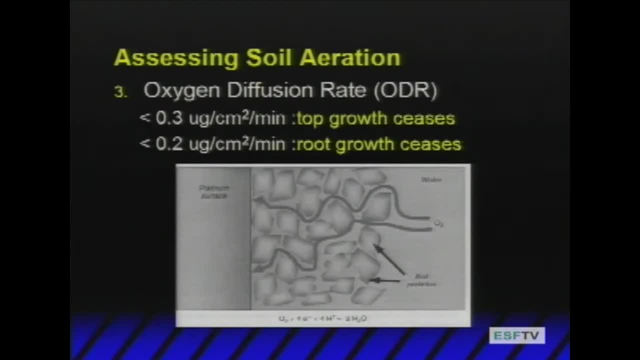 and because of the differential in voltage across those electrodes, we can actually measure the rate. So we can measure the rate of diffusion And the general numbers are. look at those units We have if you're less than about 0.3 micrograms. 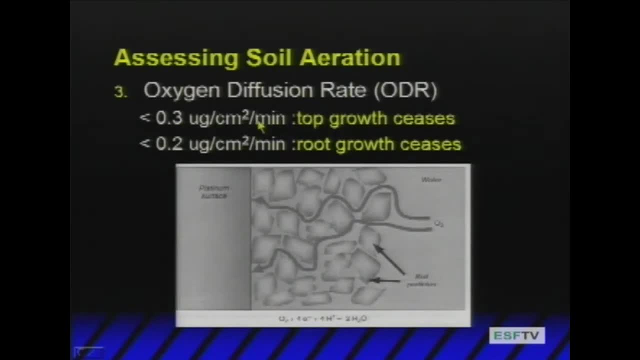 per centimeter squared per minute. that's the loss of top growth. Okay, so this diffusion rate has a concentration, micrograms, an area centimeter squared and a time minute. So this is a diffusion, It's a rate amount per unit area, per unit time. 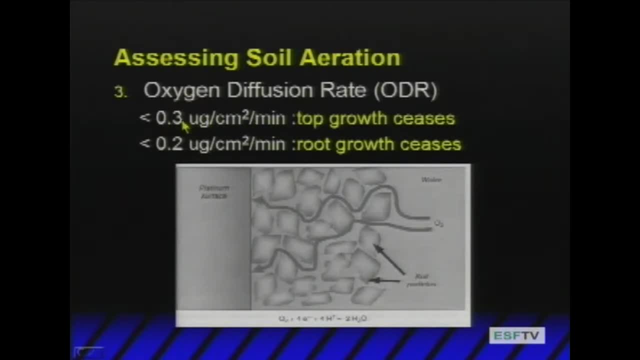 And so these numbers 0.3 and 0.2, these are threshold values So we can measure this diffusion rate. put these platinum electrodes in the soil and if it registers less than 0.3, around 0.3 to 0.2 micrograms per centimeter squared per minute. 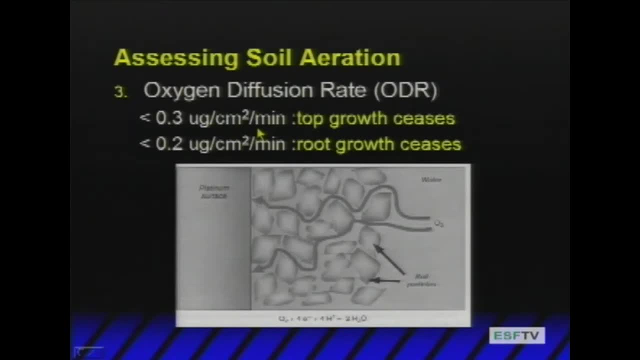 we would say that was a poor diffusion rate And so we'd say soil aeration is perhaps less than desirable. We can get these measurements, So you go to wetlands or saturated soils and sometimes you have very low diffusion rates, And this slide here depicts diffusion. 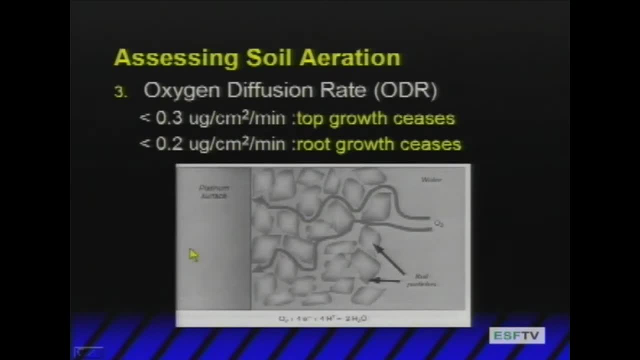 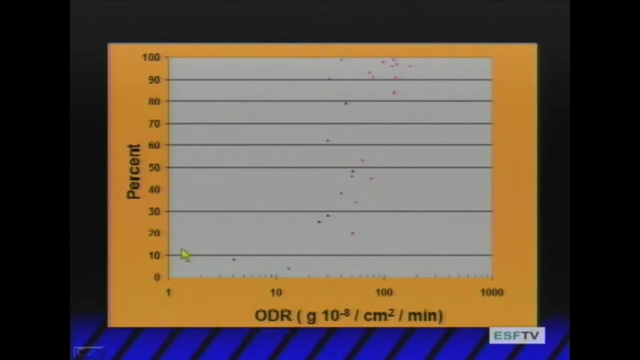 diffusion of oxygen. Here's some data from a colleague in Georgia, a couple of his grad students. Scott Toriano, one of the Larry Morris students, looked at the percent oxygen, percent growth, percent change in oxygen diffusion rate. So here's this: grams times 10 to the minus 8 centimeters. 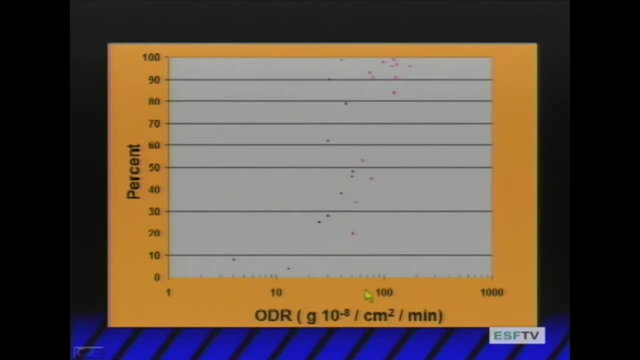 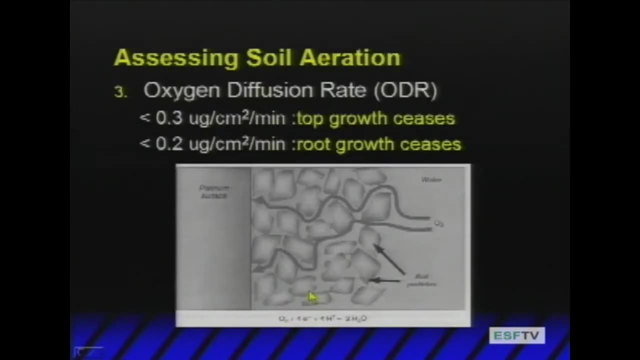 squared per minute. okay, And this is 10,000, okay, So you can relate back to our last slide And if I just go back that way, you see that 0.3 micrograms- okay, that's 10 to the minus 6, 0.3, okay. 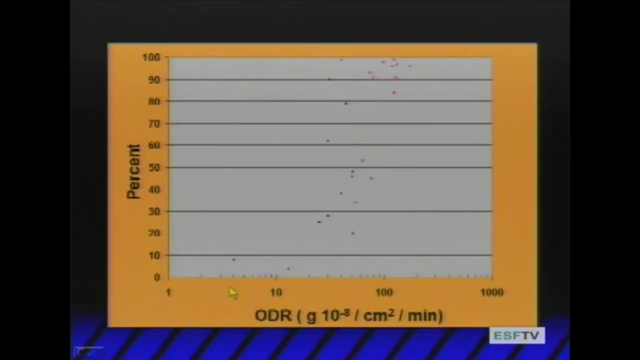 And so where is that here? 0.3 times 10 to the minus 6, so that would be 30 times 10 to the minus 8,. okay, And so we're looking right around here as that cutoff point, okay. 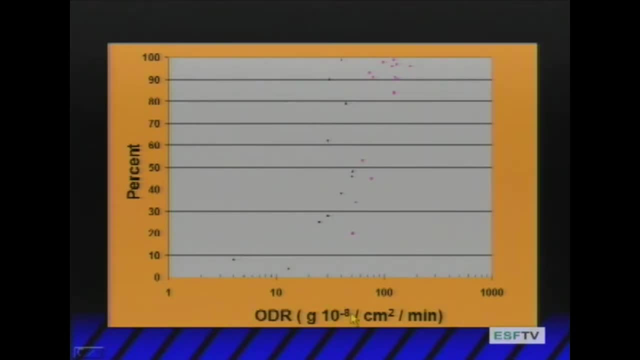 So that kind of relates this And note the scale. This is in grams 10 to the minus 8 grams. okay, And if we look at what happens with loblolly pine seedling emergence. So what Scott Toriano did was adjusted the moisture level. 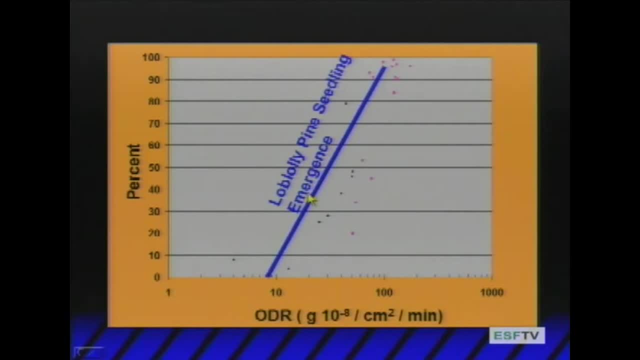 and measured the oxygen diffusion rate and planted loblolly pines And those loblolly pine seedlings didn't emerge. okay, didn't begin to emerge until we get around to that critical 0.2 to 0.3, or 20 to 30,. okay, 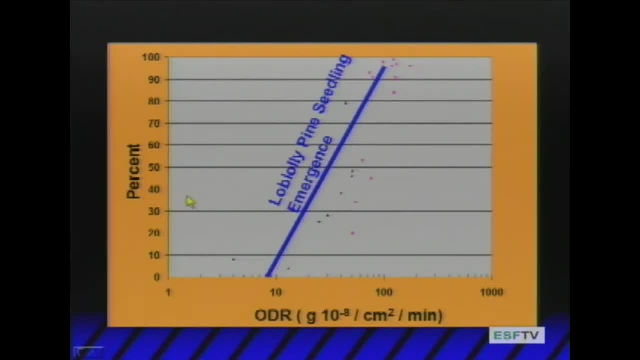 So you can see that the rate, the percentage of emerging seedlings, is very low until we hit that threshold, and then it increased linearly. So here's a nice illustration of the impact of aeration, measured by oxygen diffusion rate, on the emergence of loblolly pine seedlings. okay, 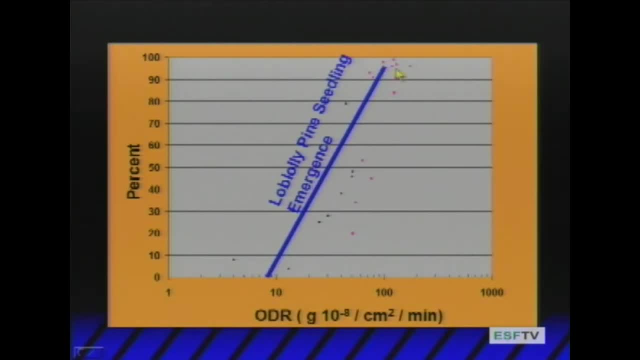 From 0% emergence to 100% up when we get up around 100, okay, Pretty nice piece of work. Now he not only did loblolly pine seedlings, but they also looked at cotton, And it's interesting. 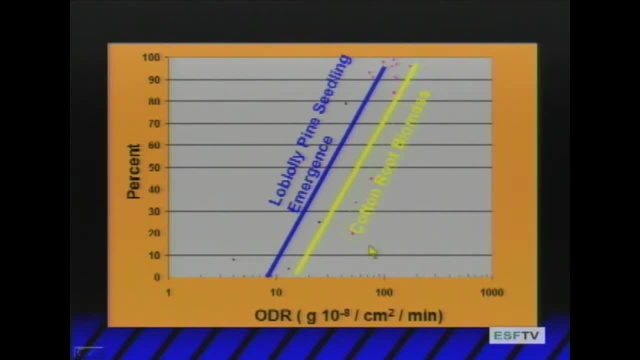 So they had cotton roots, they measured and then they measured the biomass in these various conditions And it was the same kind of a relationship. There was a direct increase of root biomass with oxygen diffusion rate, showing the importance of aeration. And again, the threshold, the cutoff. 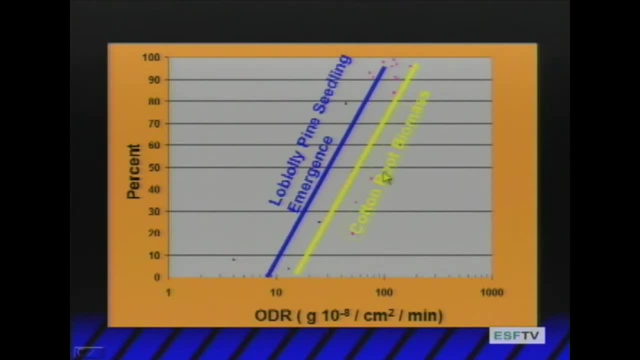 pretty close to what the loblolly pine was. So very different species, a different system. And here we're measuring seedling emergence. Here they measured root biomass, but the same kind of a slope. So this would suggest that this oxygen diffusion rate 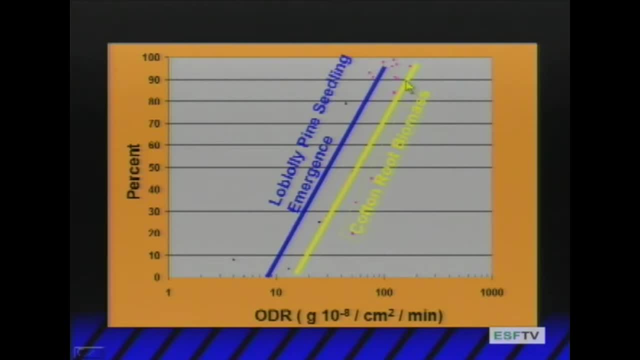 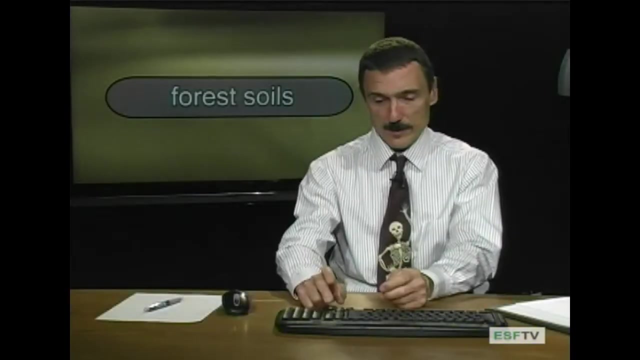 is perhaps a useful measurement to assess soil aeration, And these data from two different systems would support that. So we've had porosity, macrofil, pore space oxygen diffusion rate, And now we look at something else, Another way that we might assess soil aeration. 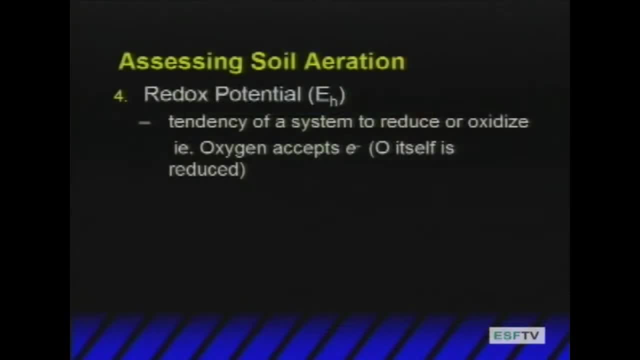 would be something called redox potential, And the symbol for that is capital E, small h, okay, And it's measured in volts or millivolts. And so what is redox potential? We can define redox potential as the tendency of a system to reduce or oxidize. 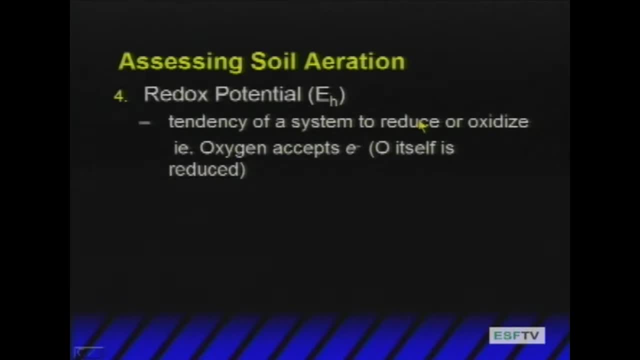 So what is reduction? So, remember, we define reduction as the gain of electrons and oxidation as the loss of electrons. So we can measure that: the tendency of a system to gain electrons or to lose electrons And, for example, oxygen, the great electron acceptor. 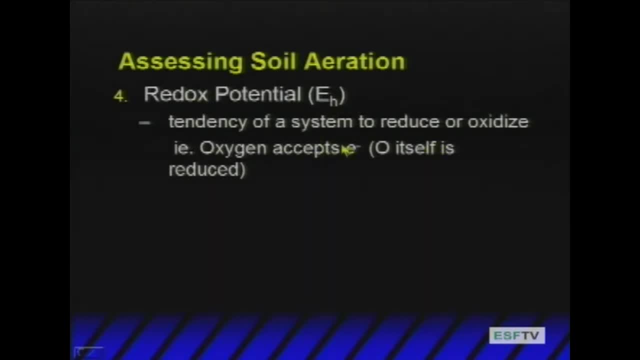 that accepts electrons and is reduced. Okay, so oxygen is something that we use to oxidize, but electrons flow to oxygen And so in this process oxygen itself is reduced. So you can't separate out oxidation and reduction If something is oxidized. 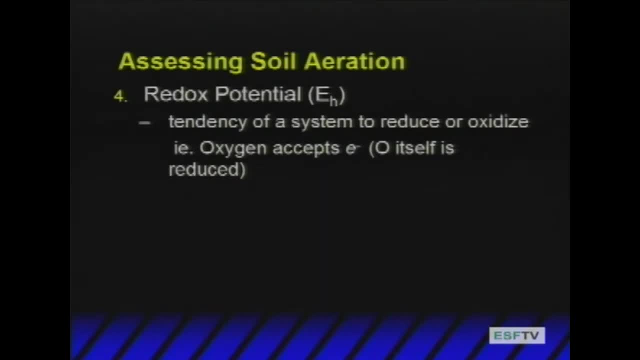 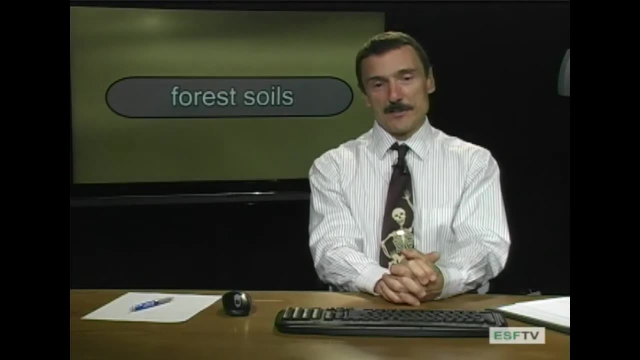 something else has to be reduced. Electrons just don't disappear. They're either. they go somewhere, They're either gained or lost. What happens when oxygen is not available? Okay, those we talked about anaerobic systems. Dissolved oxygen is not present. 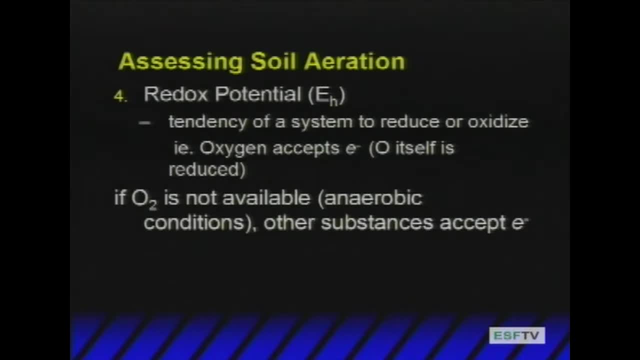 Then there are other substances that take on these electrons, So the biota continue to try to generate to respire. then respiration shut down and so anaerobic respiration. some other processes occur and electrons build up, And so the electrons no longer flood oxygen. 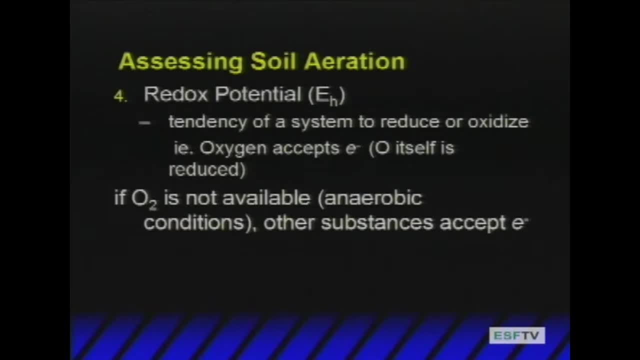 Oxygen is no longer there. So where do these electrons go? Well, the question is first, where do they come from? So you remember glucose, that six-carbon sugar that everyone knows and studied probably back in cell phys, in cell bio glucose. 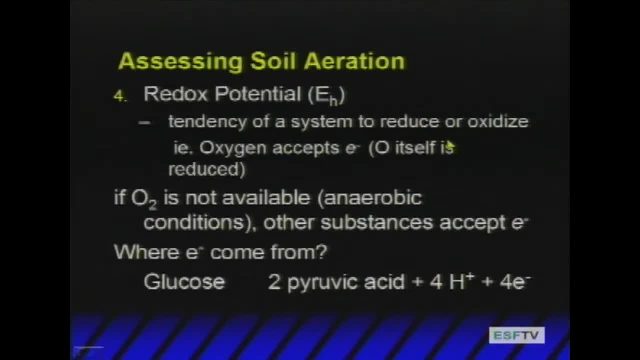 Glucose gets converted in respiration to pyruvic acid and H+, and then the process generates electrons. So this process of generating energy, okay, and respiration generates electrons, And so these electrons have to go somewhere. They just can't disappear in the system. 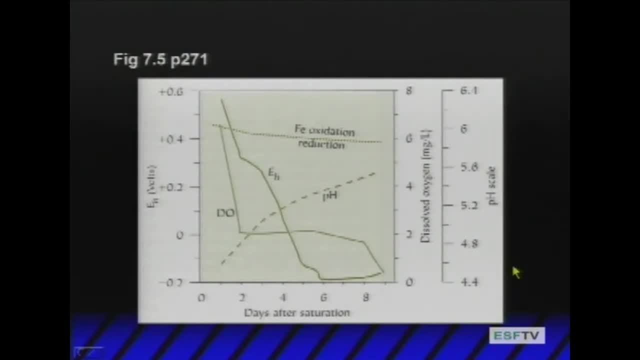 And of course they go to other things. So if oxygen is not around, they go to iron. So here's a nice illustration showing this measurement of redox potential. Here's Eh on the y-axis and here it's measured in volts. 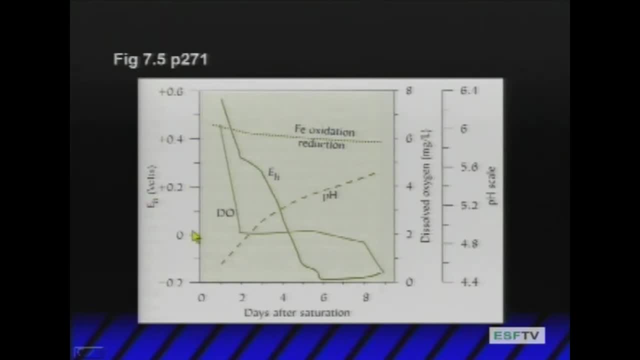 And note the scale. We're going in tenths of volts, okay, and zero positive, and we go negative, and then minus .2,, minus .4,, minus .6.. And we look at days after saturation. So essentially what happens after a rainfall. 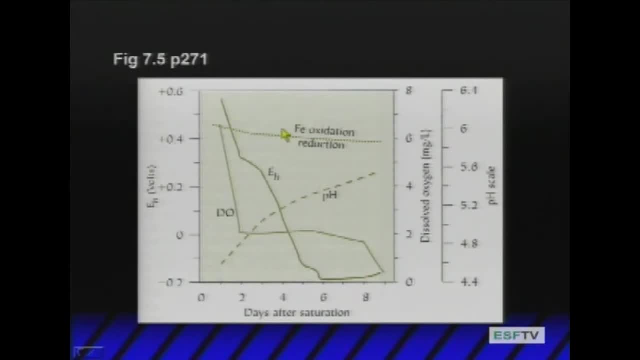 And so here's the measurement of iron oxidation versus reduction, And here is Eh After a rainfall. they're very saturated. We start after saturation. We start with a very. The Eh drops precipitously, okay, Okay. so what happens after rain? After rain, all the plants are looking for oxygen and everything's stopped. All those pores are filled with water, So immediately the process of respiration generates all these electrons. They've got no place to go And the system goes from a very positive Eh. 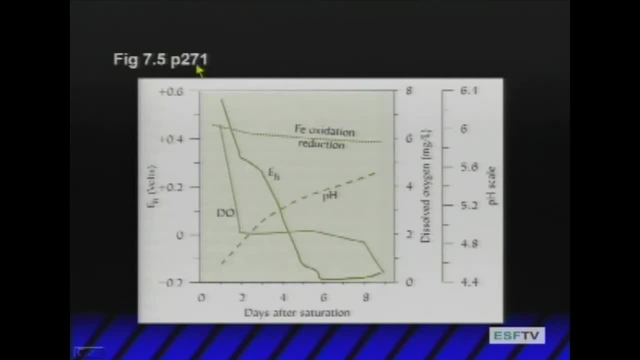 to a very negative Eh. So it's a very precipitous drop. The same thing occurs. Look at dissolved oxygen, Dissolved oxygen drops. Here's dissolved oxygen on the right. Okay, Dissolved oxygen drops precipitously along with Eh. 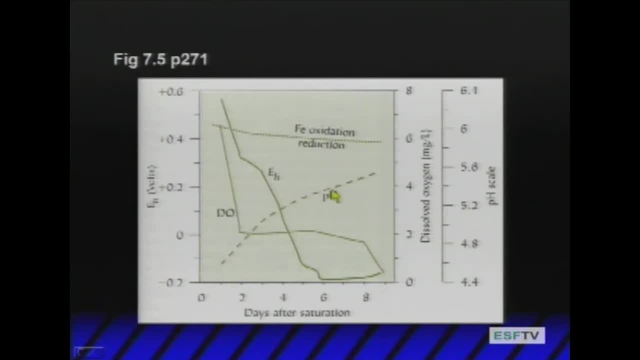 And what happens with pH. We'll discuss pH next week. pH, the hydrogen ion concentration, negative logarithm, But during the system, when that happens, the pH increases. So a very dynamic system as Eh is going down and dissolved oxygen going down. 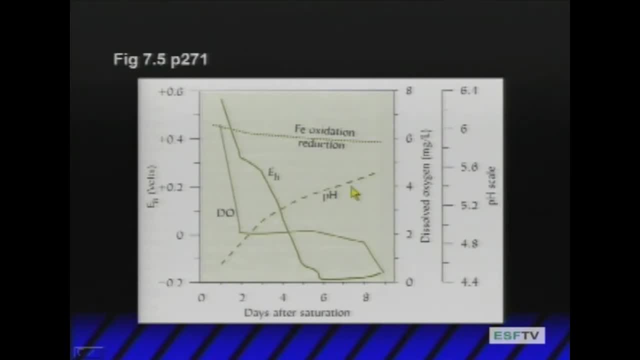 pH is going up, And so it creates a very complex relationship of electrons being generated, electrons moving, being oxidized and reduced. Note what? Let's go back to our Eh. So we go down the Eh, We've got the system. 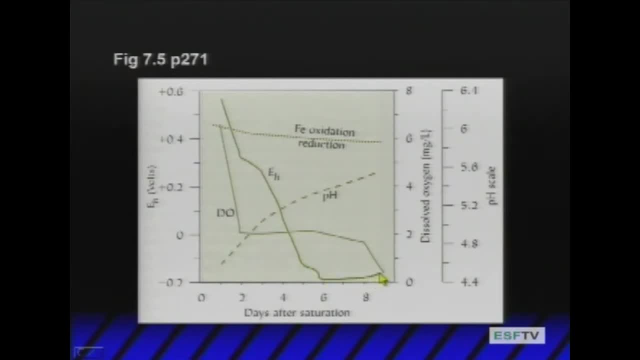 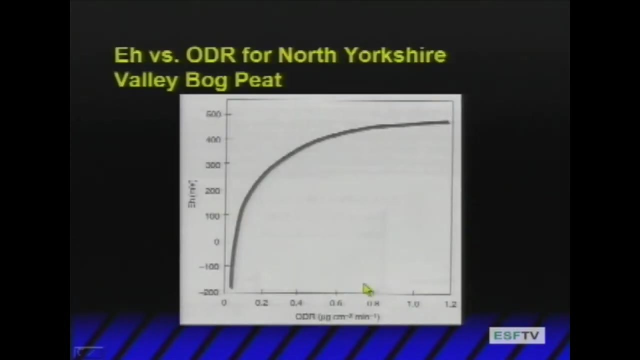 It's rapidly All the dissolved oxygen use up And then, as the system begins to drain- okay, six or seven days here- we start to see a great improvement in the situation. okay, The soil drains and the Eh climbs back up. 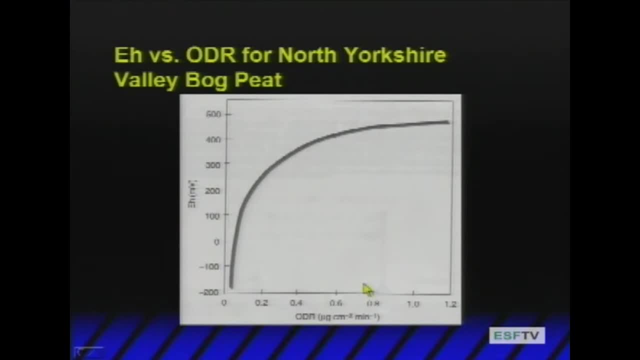 So let's look at the relationship between Eh and oxygen diffusion rate, And here's a peat bog. So here we have oxygen diffusion rate, okay, 0.12, and it's micrograms per centimeter squared per minute, And remember 0.3 and 0.2,. 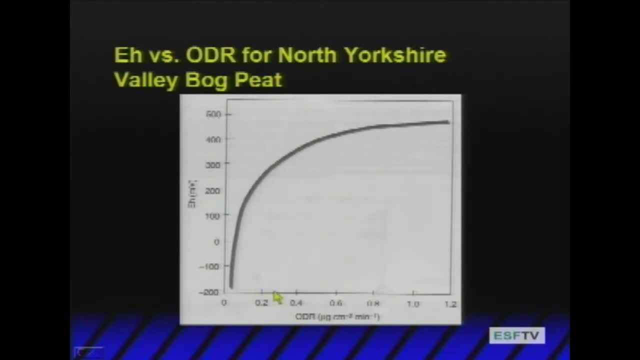 those are the cutoffs for poor aeration. So as the oxygen diffusion rate becomes higher, okay, the rate becomes greater, the Eh becomes greater. So you start to see a relationship between these variables that we've used to assess aeration, And they're correlated. 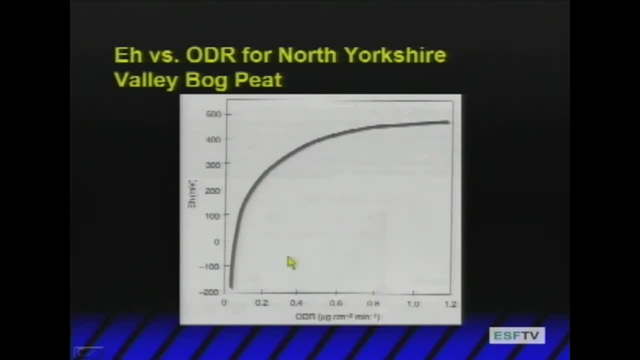 As Eh increases. oxygen diffusion rate increases As Eh increases. dissolved oxygen increases As Eh increases, the macroferocity increases. So all these numbers, they're related And we could maybe use one or another of them to assess soil aeration. Any one of them might do. Some are more common, Some are more difficult to measure. The platinum electrodes for oxygen diffusion rate are very finicky and difficult and that's a tough measurement. But the probe for oxygen and CO2 is very simple. 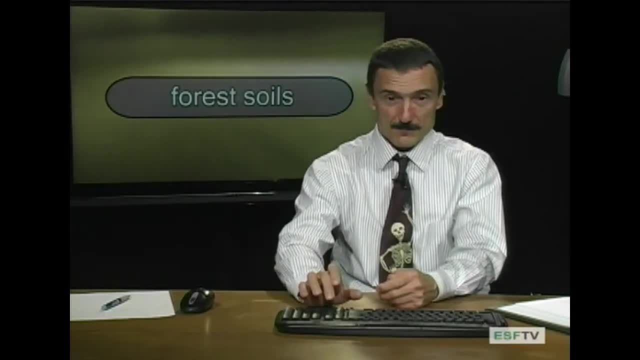 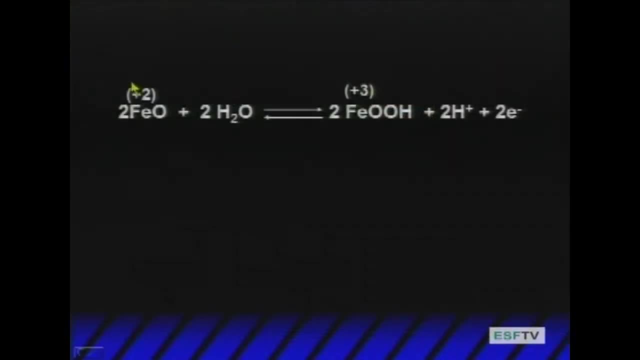 and that's a very easy measurement to get. Let's look at the process. So we have in this, we have iron here, the plus-two valence and it's going to plus-three okay, So what's this process called? 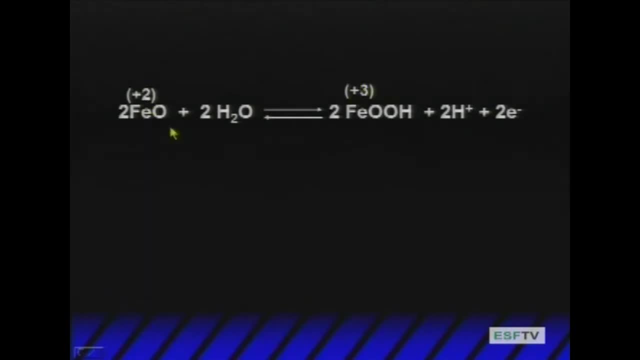 We go from a plus-two to a plus-three, We lose electrons. That is oxidation, And in the process we generate electrons, Those electrons have to go somewhere. So where do those electrons go? Okay, they don't just disappear, And here's an example of what happens. 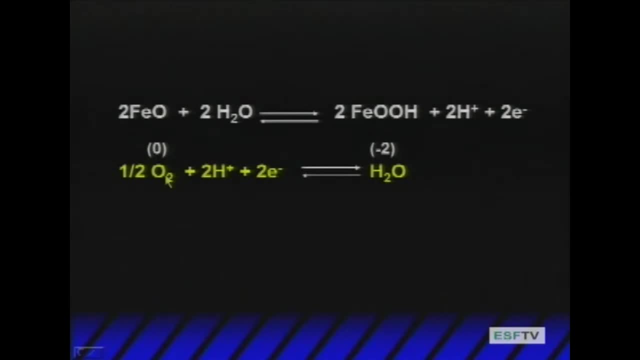 Oxygen accepts the electrons. So we have this oxygen, this half mole of oxygen with hydrogen, and it accepts this electron. and now we have water. So oxygen itself is reduced to water. Okay, so iron, FeO plus-two, going Fe plus-three. 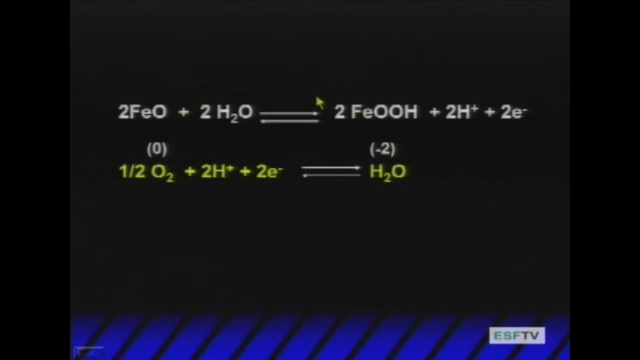 that's oxidized. So that oxidation is due because the electrons flow to oxygen, And then we make water And of course water is the reduced form of oxygen. So it's a fairly linked system. One thing occurs and not in the absence of the others. 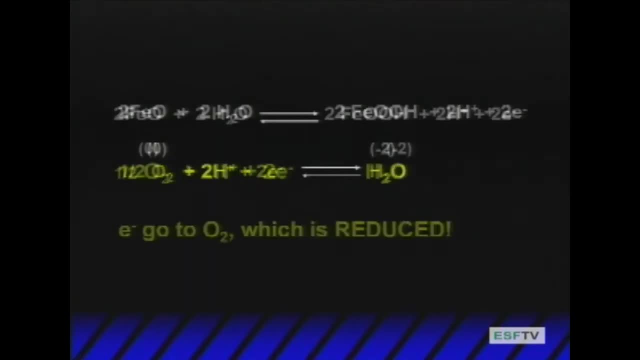 Oxidation reduction is a paired reaction. So when you see that, when you see that oxidation of iron, you see it written this way in the textbook And we talked about how iron is oxidized and we talked about weathering, I think we used this example. 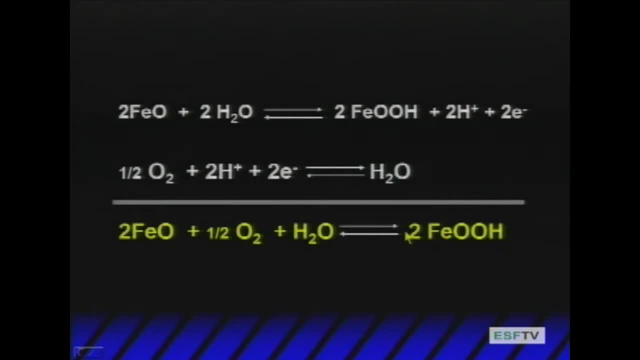 FeO going to FeOOH. Okay, so this: we didn't show all those electron balances, the electron transfer, But now we show that explicitly to make the point that the electrons that are lost from iron go somewhere and they flow to oxygen. 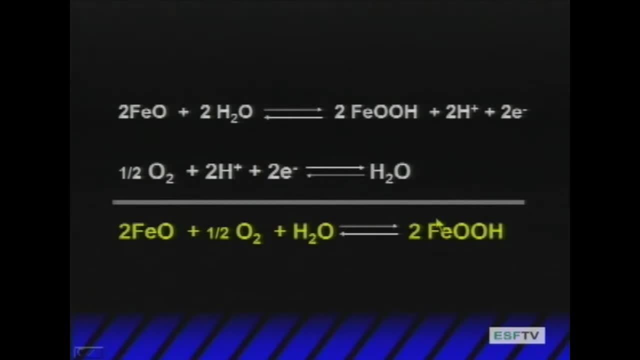 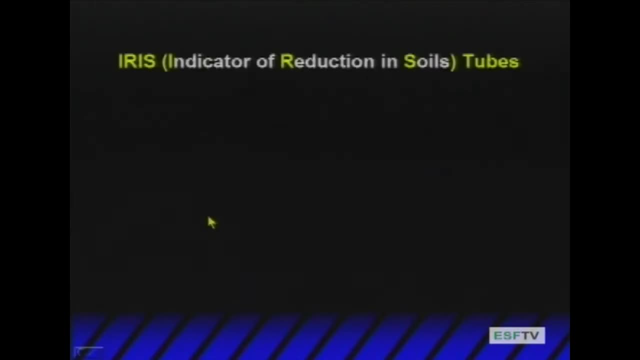 So in the presence of oxygen, iron is oxidized. That brings us into another way to evaluate these aeration status And we can think about trying to look at reduction. And so actually Marty Ravenhorst and some colleagues down in Maryland devised a very interesting method. 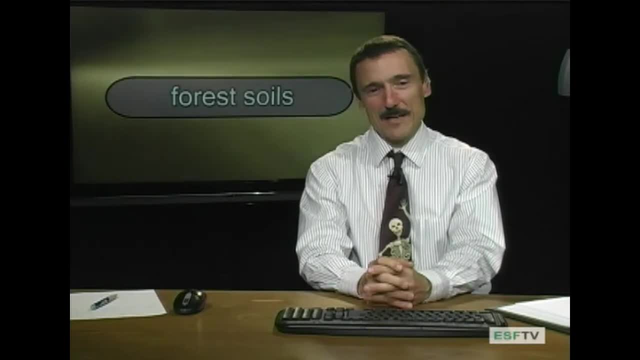 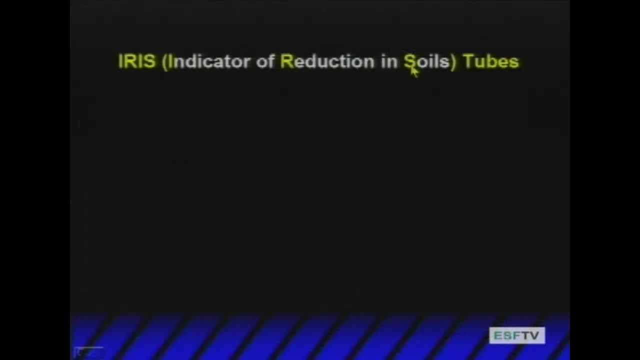 to evaluate aeration status, They devised a very interesting tube called the IRIS tube, And IRIS is short for Indicator of Reduction in Soils. So these are tubes that are actually painted- PVC tubes painted with an iron compound. And here they are. 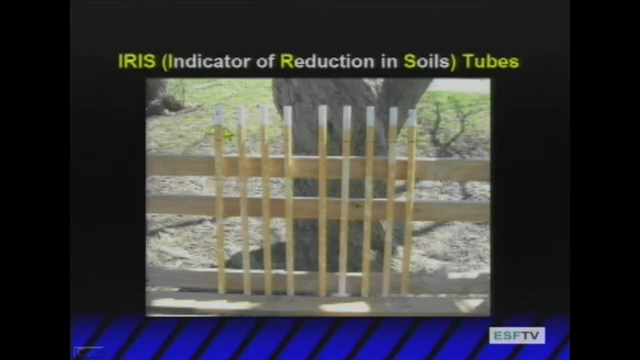 So this iron compound is yellow And these tubes. we had an experiment out near the Seneca Falls, Montezuma, and looked at reduction, So these were placed in a wetland And what happens is that when you put these tubes in the ground, 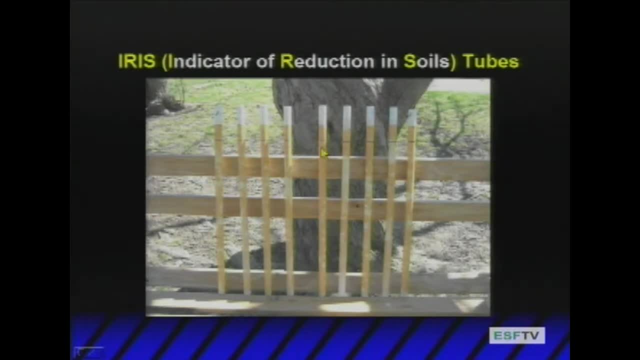 the iron is reduced and reduced iron turns gray, And so we can actually quantify the area. Here's some orange iron and then gray, So you can actually use this to quantify and demonstrate reduction simply by a change in a paint pigment of a buried tube. 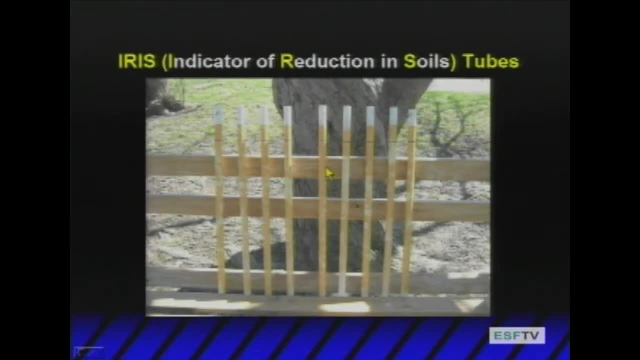 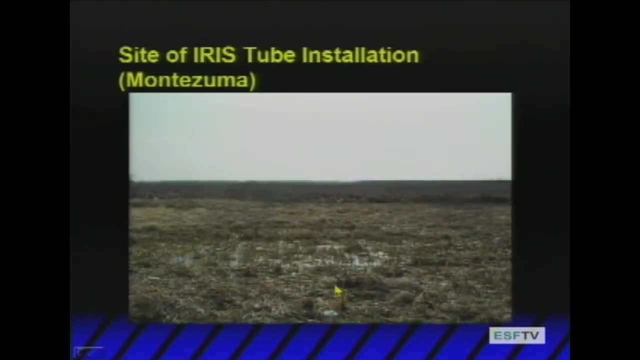 You put these tubes in for a couple of weeks and pull them out, and it's a nice way to demonstrate reduction. Here's a picture of that in Montezuma, these installations. This was a field trip we had last year in a very pronounced wetland. 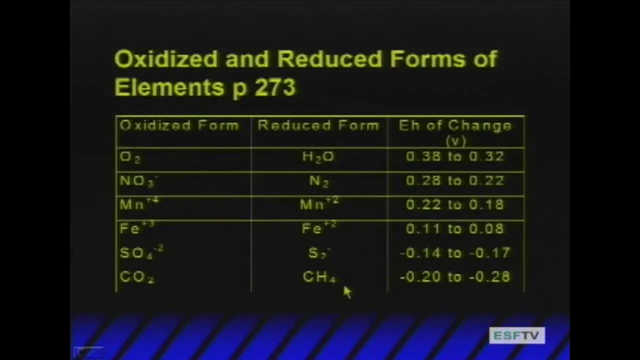 It's continually saturated, Place these tubes in, And so now we've got the picture, let's think about what's actually happening. So here's a table from the text on page 273 on oxidized and reduced forms of elements. It kind of gives some a little more feel. 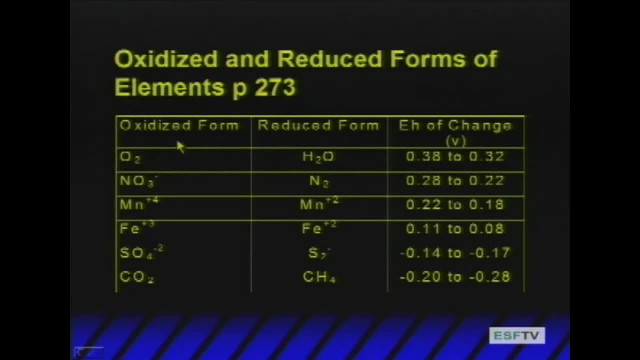 a little more understanding for what's going on. And this shows two things. It shows the oxidized form- here's oxygen. then it shows the reduced form- here's water. Now we just demonstrated that. we just showed how oxygen gains electrons. 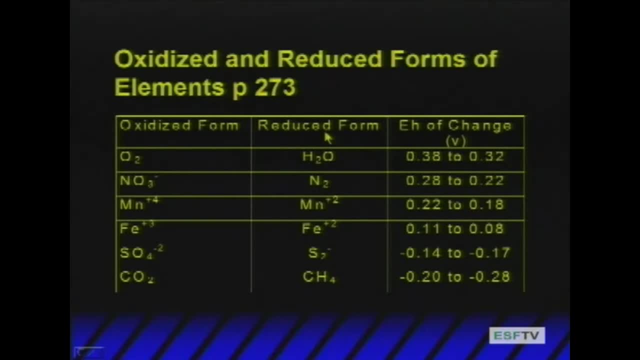 and is reduced to water. Now we can also measure the potential, we can measure the E-H. at what that happens And that change of oxygen to water takes place at an E-H of .38 to .32 volts. .38 to .32 volts. 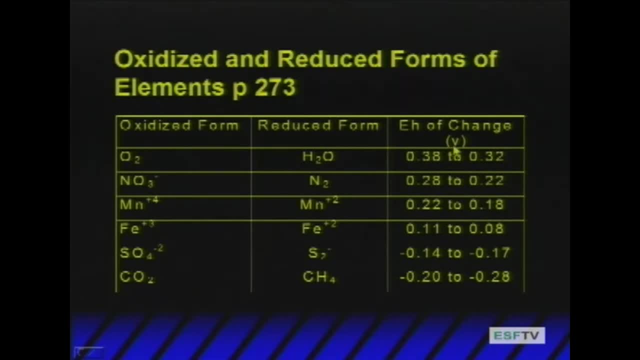 Now these are volts. if we had measured that in millivolts, it would have been a thousand times that, or 380 to 320. So something like that. Sometimes you'll see this measured in millivolts, But oxidized, reduced. 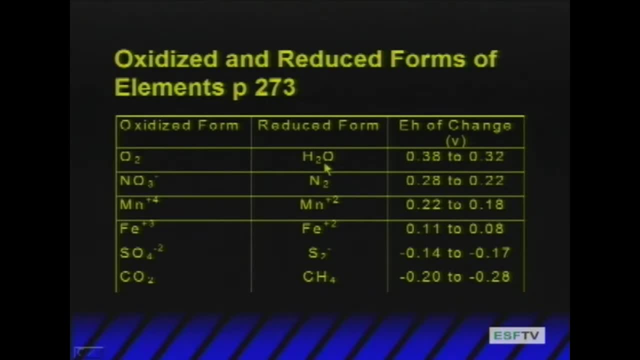 that takes place. the E-H is somewhere at .38 to .32.. Now what happens? What happens when all this oxygen runs out? It's depleted, the roots have used it all up. There are other things And at that point there are other materials. 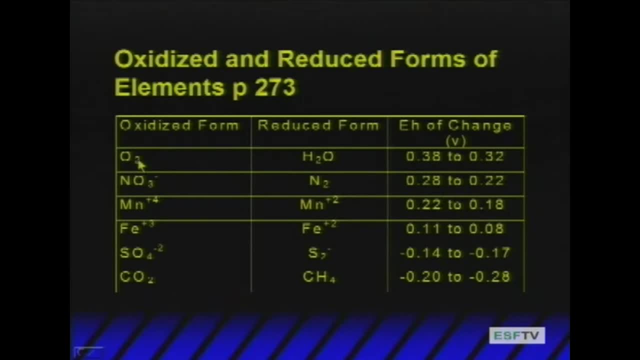 other elements that accept electrons. So after all, the oxygen is depleted. nitrate NO3 minus accepts electrons. It's reduced to N2, gaseous nitrogen. Here's a process called denitrification. we'll talk about later, But this is a very important function of wetlands. 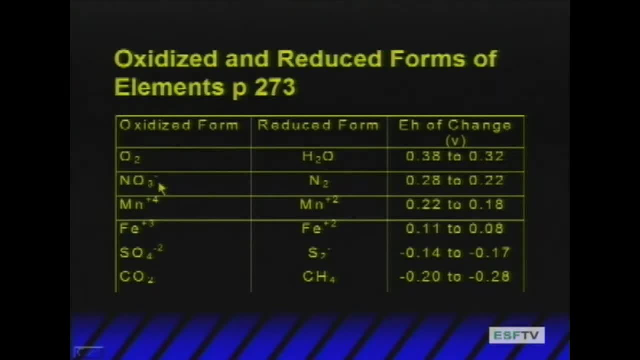 Nitrate in large concentrations is toxic. It's a plant nutrient, But this is one way that nitrogen is removed from the biological systems in wetlands and it turns to gas. So this takes place at an E-H lower E-H than O2.. So this takes place. 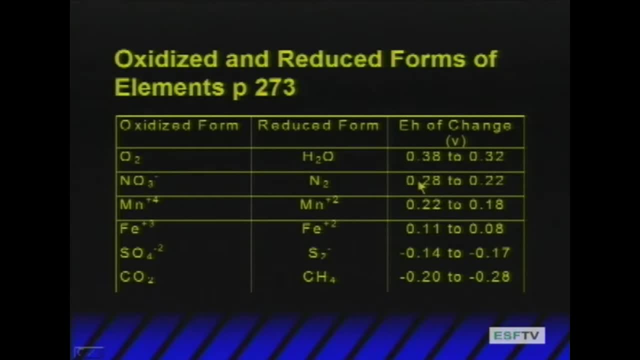 .28 to .22.. So suppose then we had these processes going on and we utilized all the nitrate, convert that all to N2.. What happens next? The next thing that accepts electrons is manganese. So manganese is reduced, goes to minus 2.. 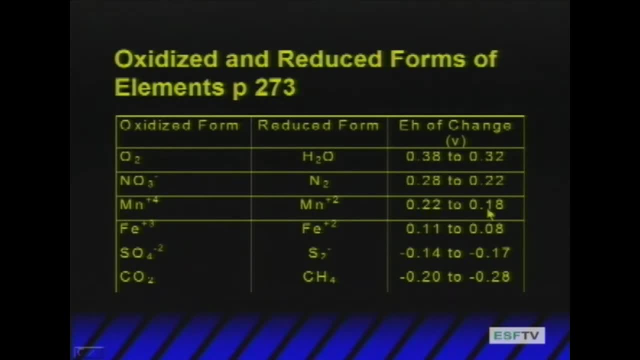 And that's in the E-H of .22 to 0.18.. Eventually all the manganese is reduced and when that happens, iron plus 3 goes to iron plus 2. And that's reduced .11.. This is the E-H range, the lower E-H range yet. 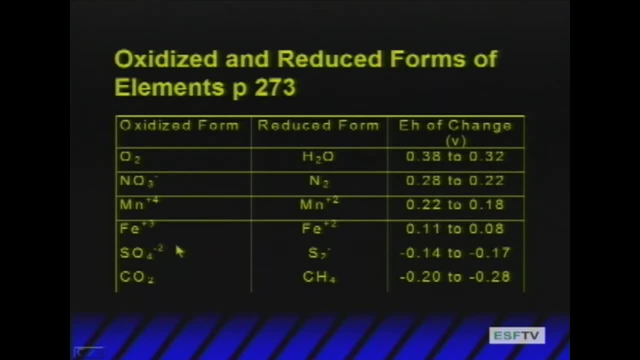 And now, when all that's done and the next thing that happens is sulfate SO4 minus 2 goes to sulfide S2.. And what happens? that's a very negative E-H. And when all the sulfate's utilized that way, the next thing that happens is: 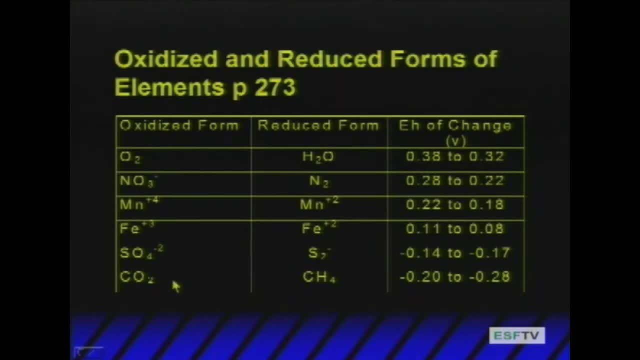 carbon dioxide is reduced to methane. So here we are in a very anaerobic system. All these other things have been reduced and now we're down to carbon dioxide, to methane- very negative. So this is very, very, very poorly aerated soil- very negative. 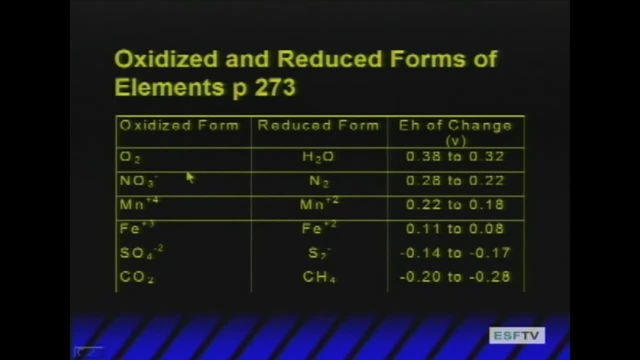 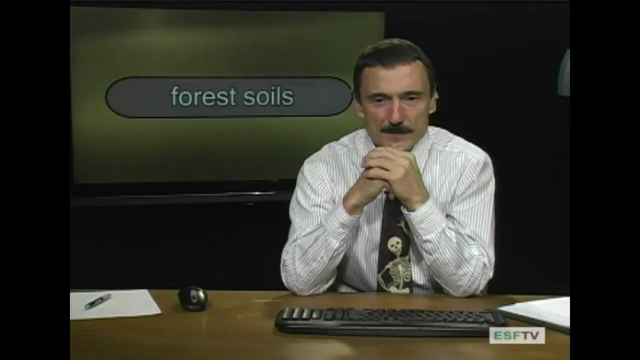 E-H And it shows the progression of decreasing potential and which of those species of elements accept electrons. So there's an awful lot in that graph And it kind of encompasses or encapsulates, summarizes all the things we've just talked about. That's a lot to swallow and probably a good thing. 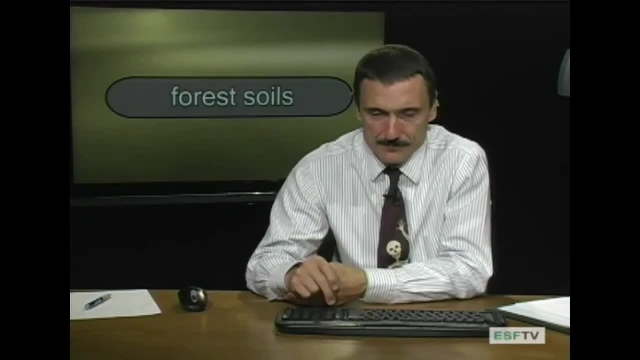 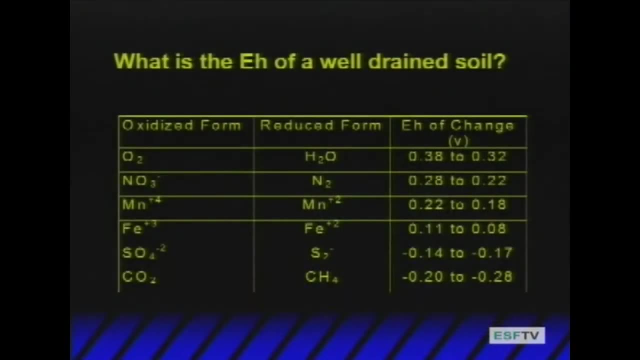 to think about. That's an important point. Now, if we're going to use this number, this E-H, this potential to indicate a well-drained soil, what number would we choose? So we look at this chart and try to think about that. 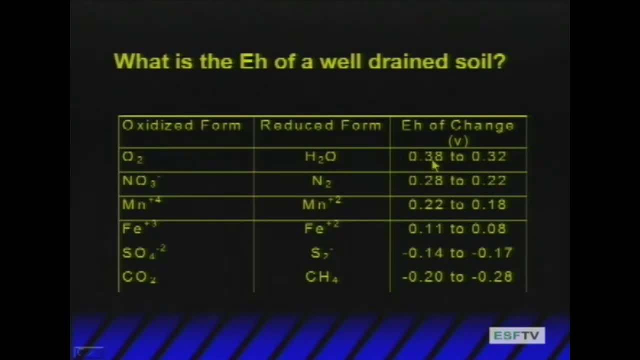 We have O2 being accepting electrons 0.38 to 0.32, then nitrate, then manganese and so forth and so on, plus 4 to plus 2.. So we look at that and we think: what number. 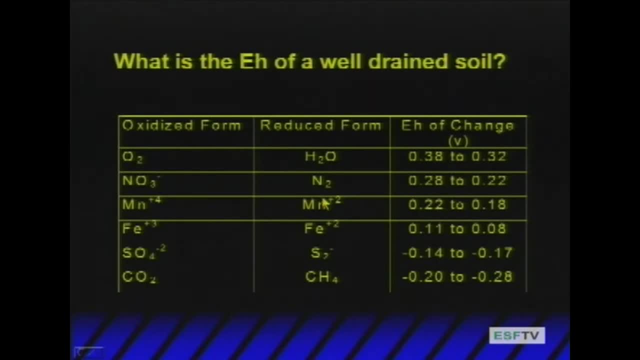 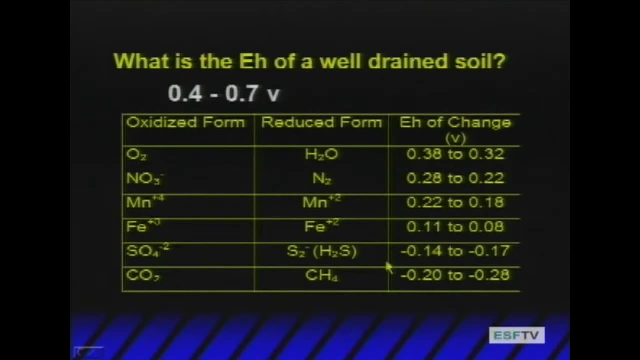 could we use to characterize a well-drained soil? Well, it certainly wouldn't be a negative number, And so the answer to that is somewhere between 0.4 and 0.7 volts. So here's our next criteria. So we had an O-D-R. 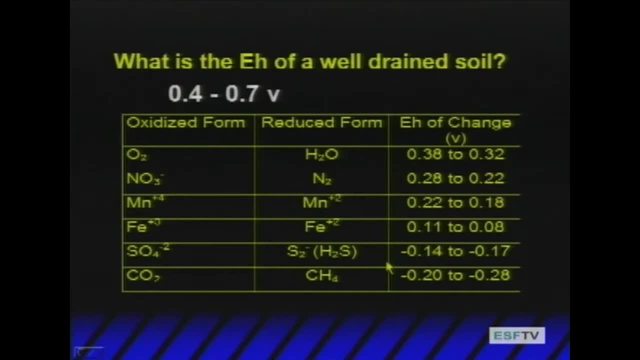 of 0.2 to 0.3 micrograms per minute per centimeter squared. per minute. We had a 10% oxygen concentration and so forth. And now this number, this threshold, using E-H, is somewhere at a 0.4, 0.7.. And given what we 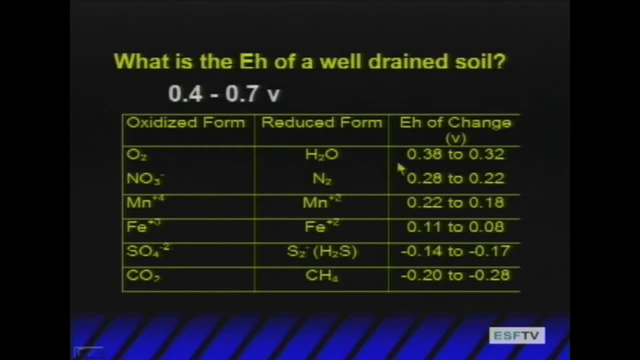 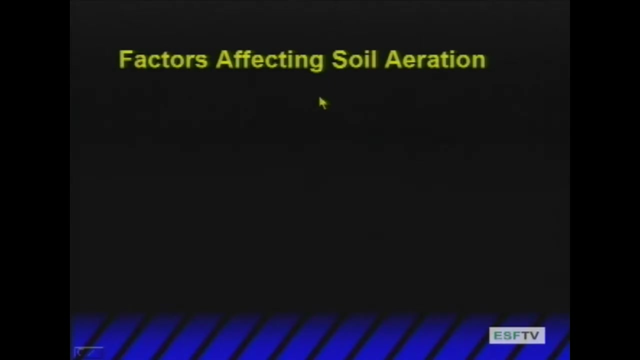 just observed here, that's just above where all the oxygen begins to be depleted. this is a reasonable number. So again, this is a useful number to know the threshold for a well-drained soil, for an E-H value. So now we've measured it. We've kind of 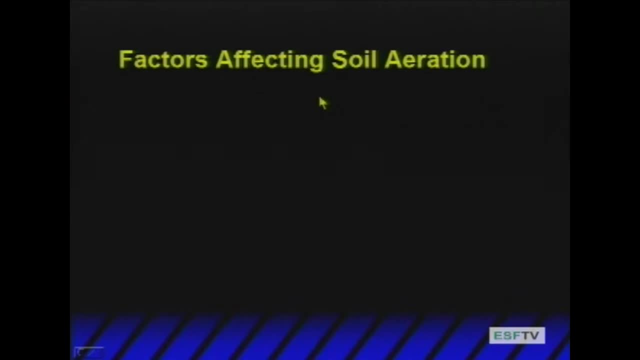 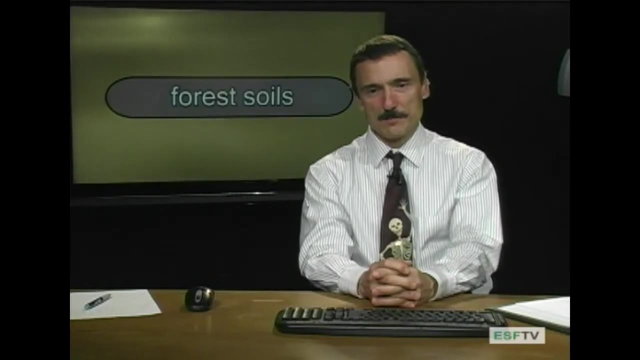 given some different numbers to indicate aeration status, And now we might go a little further. It's probably useful for us to think about the factors that affect soil aeration. if we wanted to predict soil aeration, And then we could actually link. 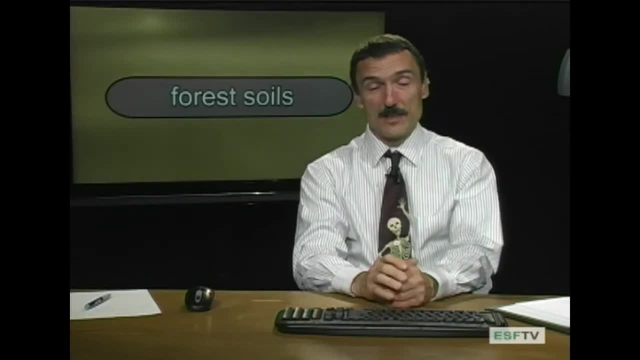 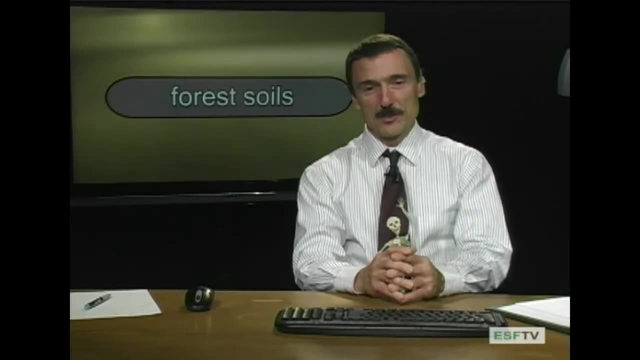 this back to our soil physical properties and our water. And again we're building on that first idea, this idea of this exchange of energy, water and gas constrain, the biota, And now we'll look at those soil physical factors that we think about to be able to predict aeration. 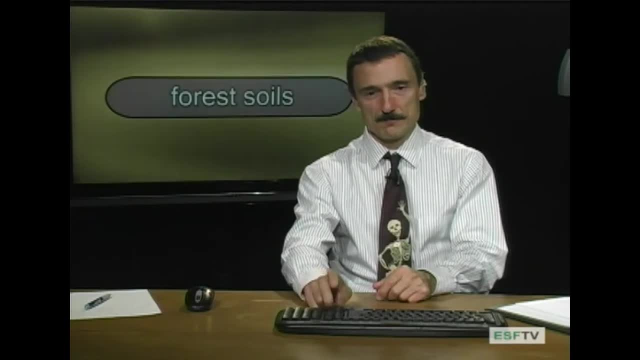 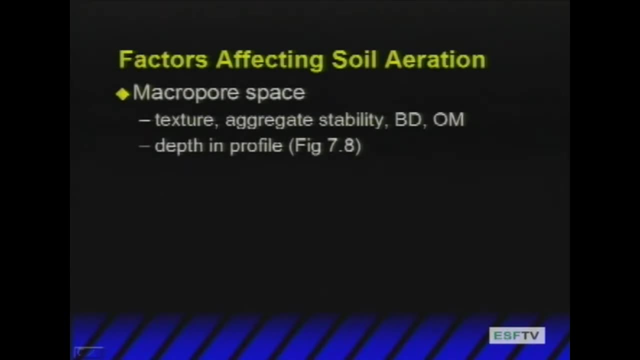 Right back to the beginning of the course And the first and most obvious- macropore space. We've seen the importance of diffusion and that diffusion doesn't take place in water-filled pores. So we talk about macropore space, And so then we say: 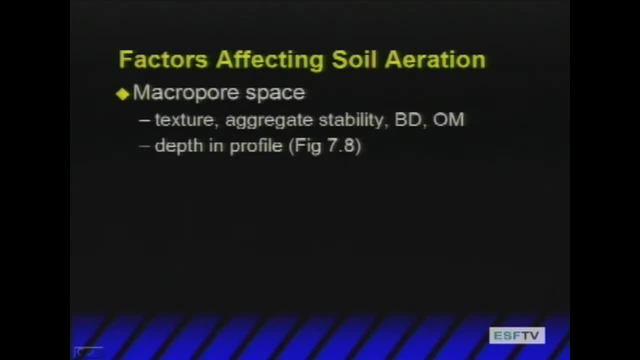 okay, what are the physical factors? What are the indicators? How do we measure or quantify macropore space? And one of those is texture, And we talked about generalizations of texture in macropore space, with sands being fairly high macropores relative. 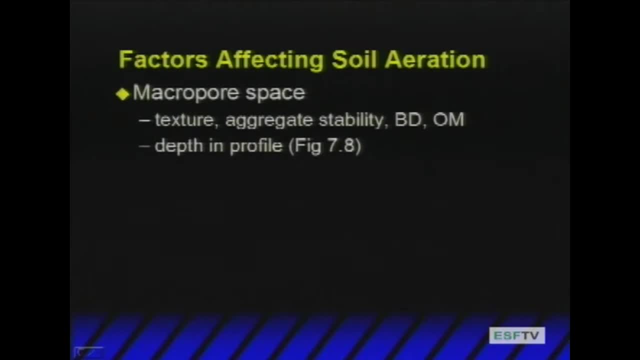 in terms of their total pore space and some of the finer textured soils being small. And then we talked about structure. Is structure modifying the effect of texture? So, again, this pipe system, going back to the original idea of the soil physical properties. 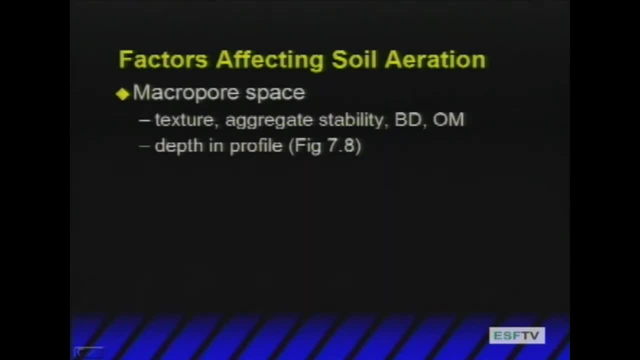 very, very important, And we add on to that we also what are the things that contribute to aggregate stability, And so bulk density and organic matter, and we talked about structure. So all those things affect macropore space And we're 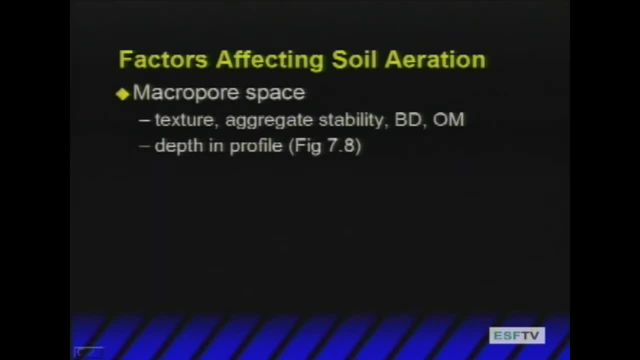 recall also that we were thinking about depth in the profile. We talked about how the exchanges of energy- water and gas- are maxing the surface and decrease with depth. So as we go deeper in the profile that macropore space is reduced, and we talked extensively. 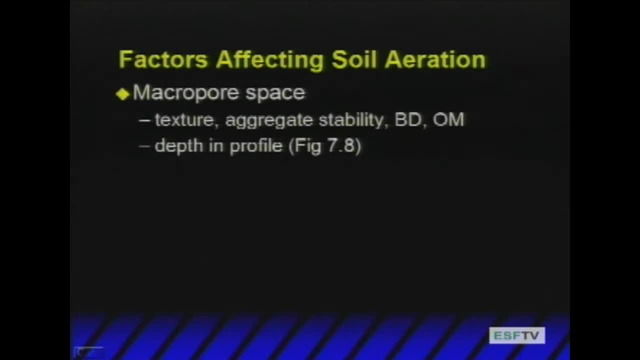 about that when we talked about bulk density and structure. So macropore space, then, is one of those prime factors that we think about for aeration, And then we could finally relate this back to our parent materials, the custom materials, the outwash materials, 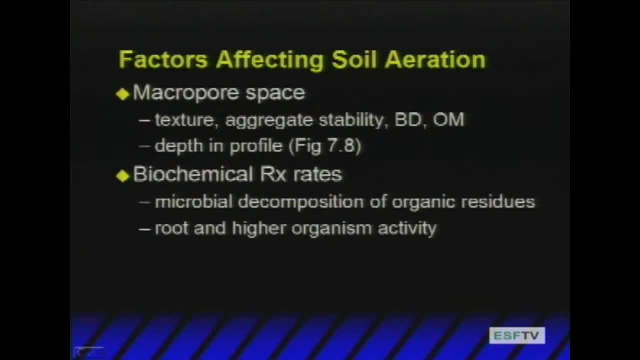 and so forth. The other thing is the rate of consumption of oxygen and the rate of production of CO2.. So the biochemical reaction rates- And this should make sense- The microbial decomposition of organic residues, the biota they churn, they chew up. 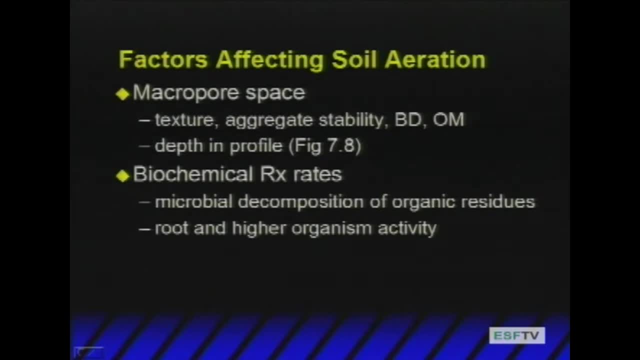 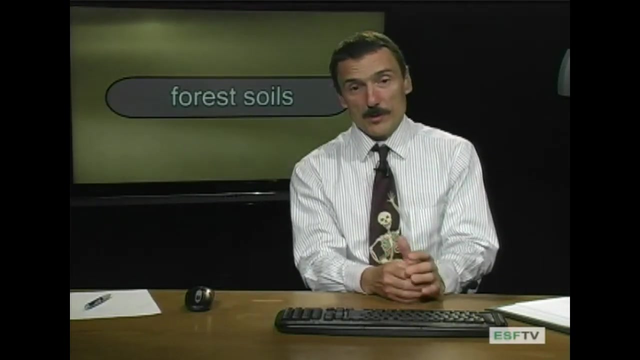 the stuff and in doing so they generate a lot of carbon dioxide. They're also utilizing oxygen for energy, So the greater that rate, the greater the need to remove that CO2 and to input oxygen. Roots are one of the more important. organisms And we think about plants. but those roots, they are very, very active. They're generating a lot of CO2.. They're producing a lot of carbon dioxide. Then there are a whole slew of biota, of fungi and microbes associated with root systems in the rhizosphere. 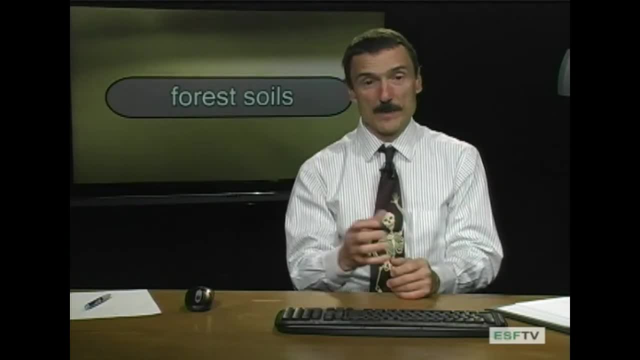 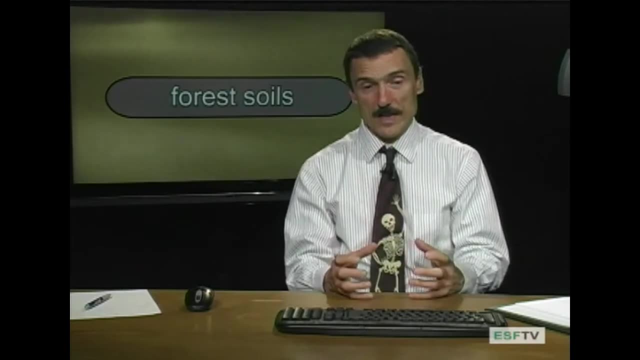 And these are doing the same thing. They're utilizing oxygen for respiration. They're generating CO2 from that respiration. So this whole biota system is utilizing these oxygen gases to generate a lot of CO2.. This exchange is critical to their 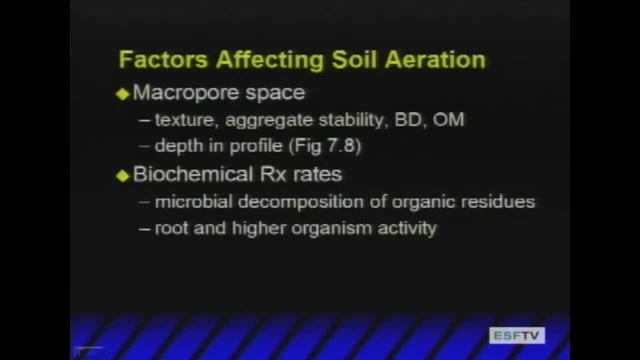 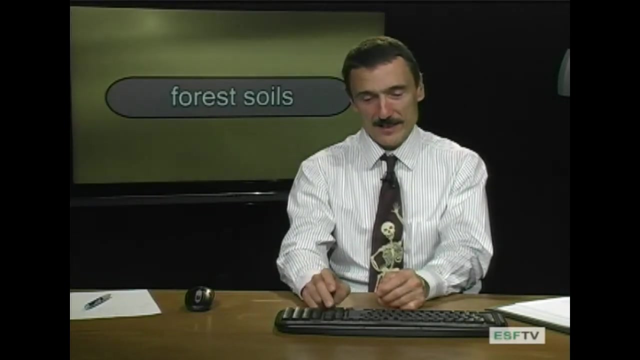 continued production Season. So season kind of goes along with both of those. We have seasonal impacts on macropore space and biochemical reaction rates, And one of the most nice, one of the nicest graphs that illustrates that is in the text with corn. 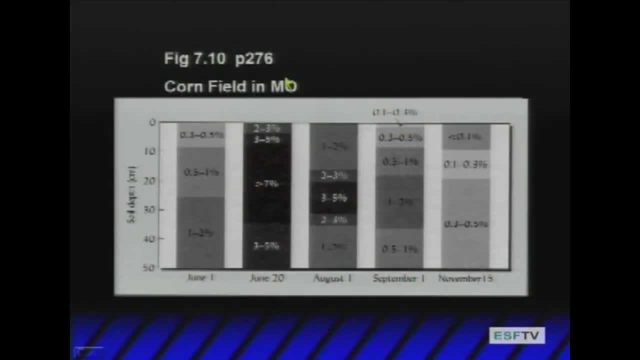 So here's a very nice illustration. So here's a corn field in Missouri And we go from June to November, So essentially the growing season, then the post-growing season of the fall And soil depth. So we're looking at the combined effect. 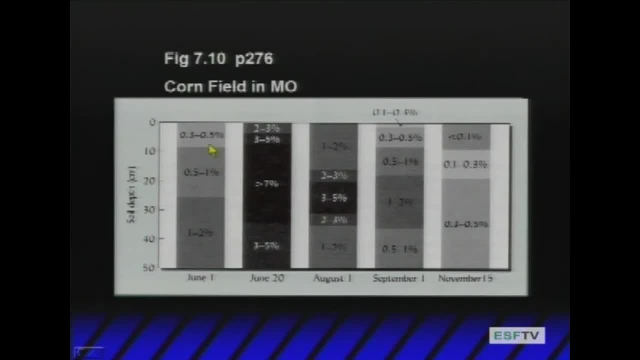 of soil depth and season And this is showing carbon dioxide concentrations. So we start out in June after planting, when the plants are just getting established, And we see the carbon dioxide concentrations .3 to .5.. Relatively high compared to a forest soil. 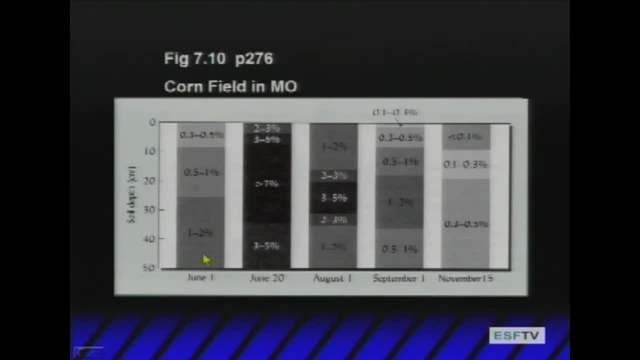 but low in an ag system, And they are increasing with depth. Okay, this is an expectation you should be comfortable with. There's less exchange. Most of the rooting activity is at the surface, But roots are developing over time, So as the growing season proceeds. 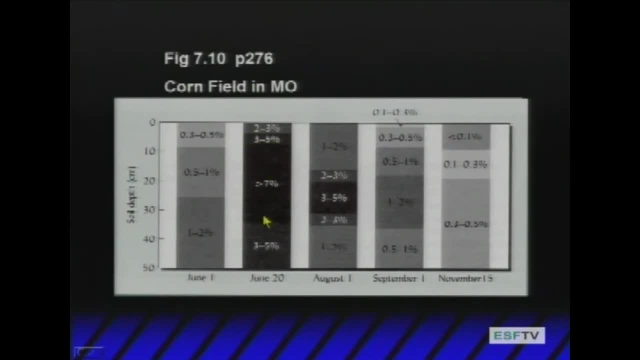 those carbon dioxide concentrations increase tremendously. Look at there: more than 7%. This is a tremendously high concentration in the middle of the growing season. The biochemical activity is phenomenal. The roots are just sucking the stuff up. The plants are growing. It's just a very intense time. 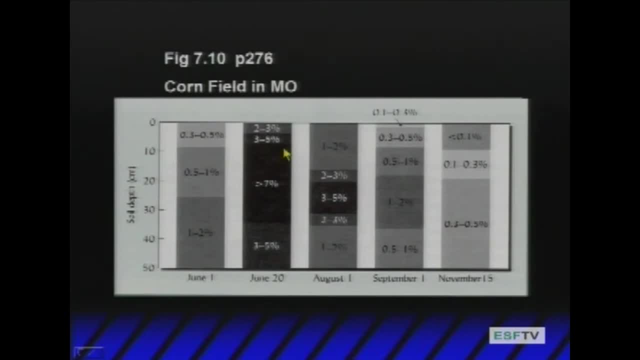 of biological activity. As we go toward the end of that growing season. the carbon dioxide is lower a little bit And they have an irregular pattern. They increase with depth and decrease. They're increasing. This depth is the maximum part of the root zone. 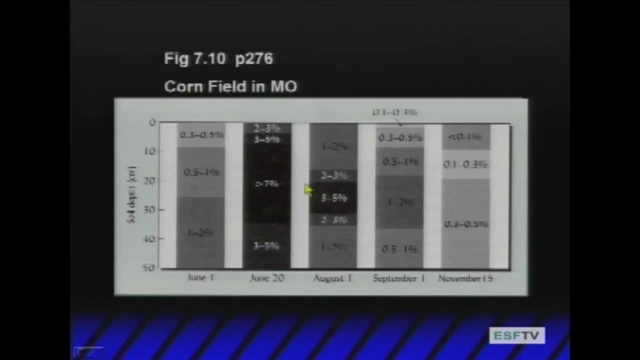 This very intense part of the root zone And then, as we go into the fall, the levels dissipate further And we go back to more of a situation of what it looks like in the spring or the early summer. Here's a nice graph. 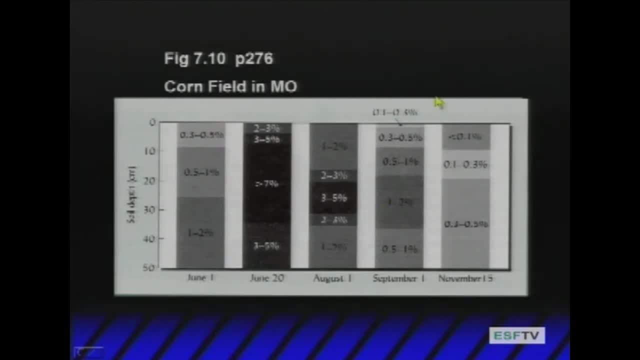 showing the interaction of concentration with season and depth. It's just a wonderful illustration of also the very high concentrations that can be attained. So you know what corn looks like. It's planted very densely- the root systems- And these concentrations are very, very high. 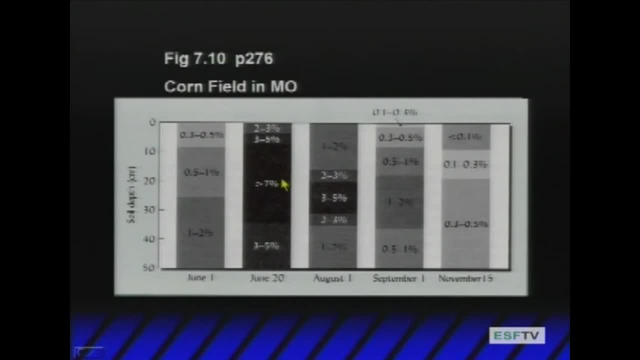 And you'll see none over 10%. Over 10% is that cutoff where aeration ceases. If they get over 10%, they're going to go down. One question you might consider. I won't answer it here, but I'm going to ask you 7%. 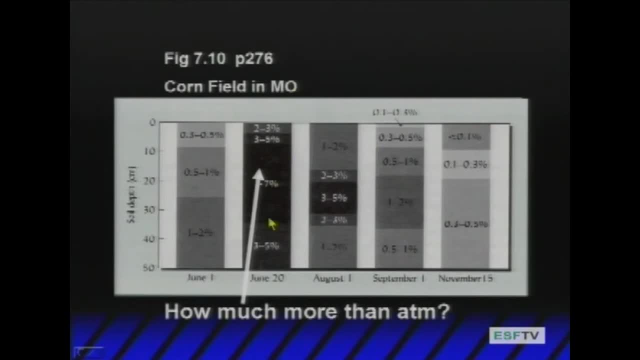 how much more is this than atmospheric? So what's the relative increase as we go from the atmospheric concentration to the soil? And we're looking at 7%? How many times greater is the concentration of 7% compared to the atmospheric? So to answer that question, 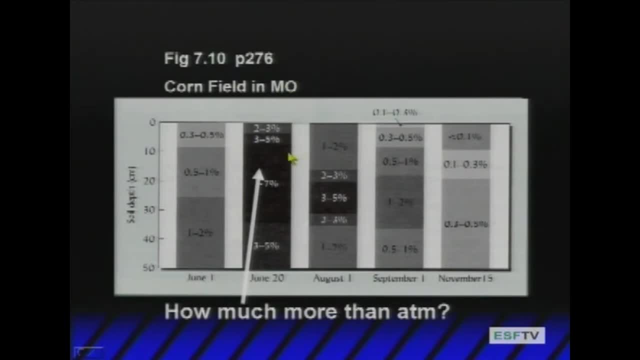 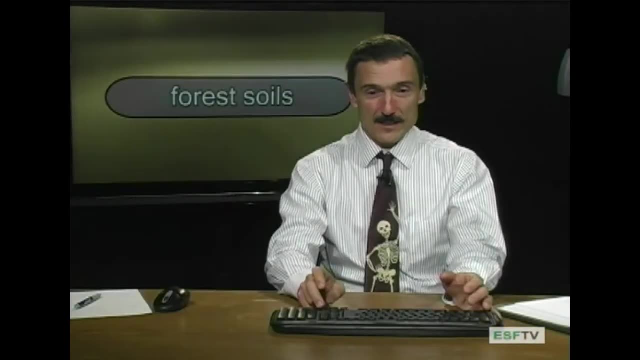 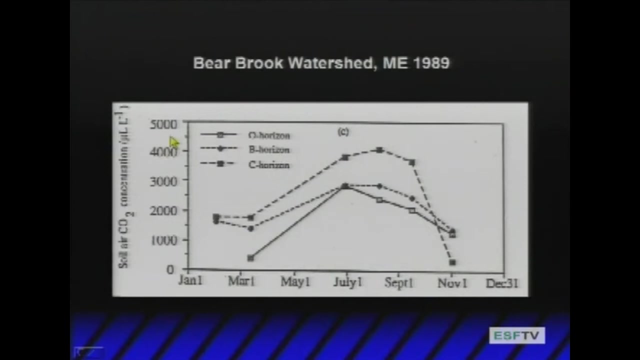 you'll have to know what the atmospheric carbon dioxide concentration is And then you have to divide, Probably on an exam. Let's contrast that. We have forest soil, So that's a very intense ag system. Let's look at a forest soil. 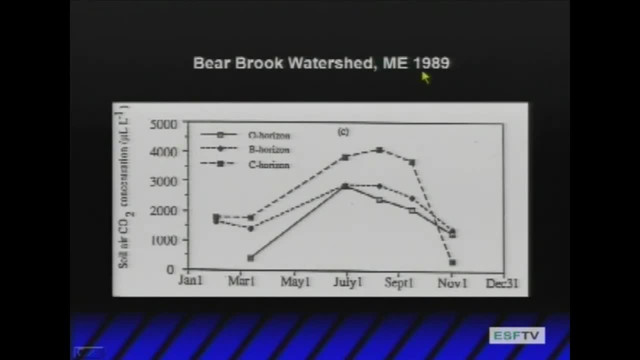 So here's some data from Bear Brook watershed in Maine. So this is some data from Ivan Fernandez from one of our gradient studies. when I was working up there at the University of Maine And we had studied the concentration of carbon, We were looking at exchange rates. 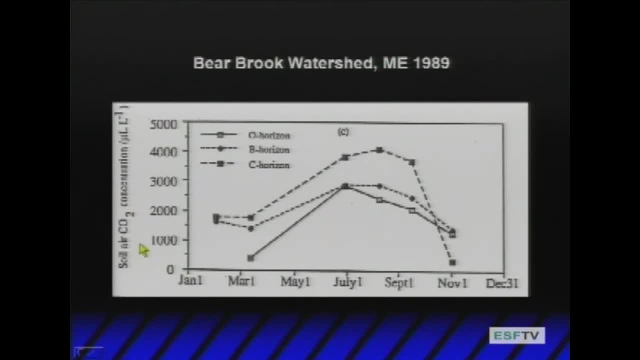 in a variety of systems across the climate gradient and we looked at the concentration, CO2 concentration, microliters per liter, or you know that, as 10 to the minus 6 parts per million, And we would go from 0 to 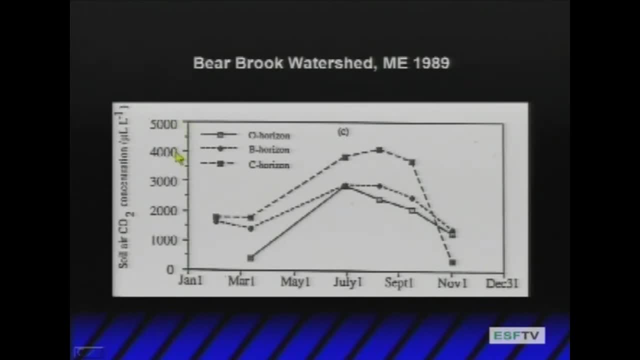 5,000 parts per million. And we also show it by horizon. So we have the O horizon, the B horizon and the C horizon And we go season. We go from January all the way to December, an entire year, And the first pattern is that the 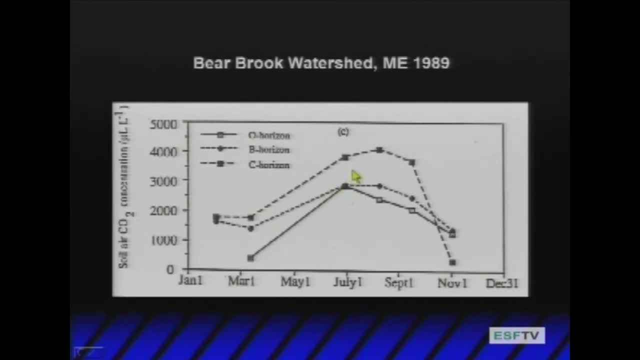 carbon dioxide concentrations are maximum just about the middle, toward the end of the summer. This is in a spruce fir stand, And the other thing is that the patterns with depth change over time. So let's look first at the O horizon. So the carbon concentrations in the 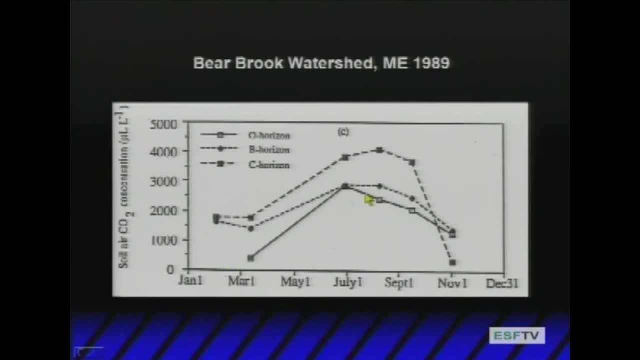 O horizon are the lowest and of course that makes sense. That's the closest to the surface And they peak a little earlier in the season And then down to the B horizon the concentrations are higher. This shows increasing concentration with depth. 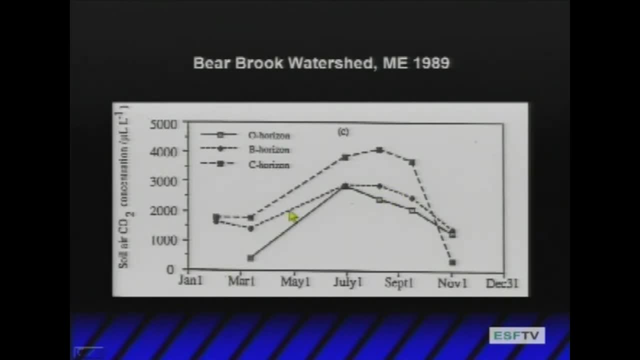 And they peak just a little bit later. And finally, in the C horizon the concentrations are higher yet and they peak later with depth. So the rates of exchange kind of lag, And so the exchange with carbon dioxide and oxygen are lowest in the C horizon. 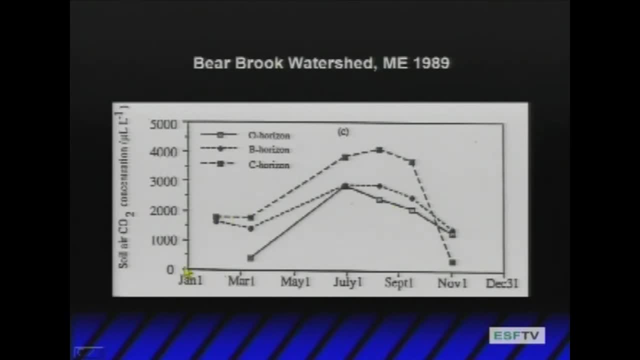 and highest in the O horizon. So look at these numbers: 1,000, 2,000, 3,000, 4,000, 5,000 parts per million, And I'm going to ask you to convert that to percent. 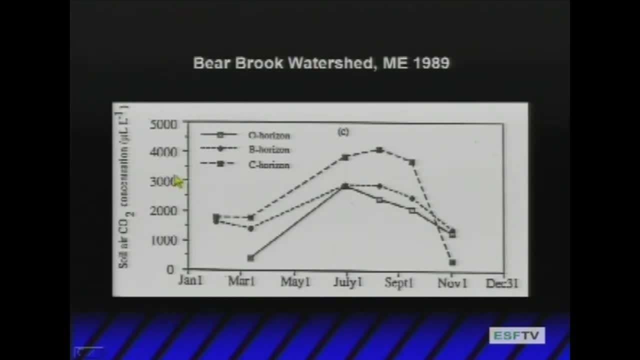 So here we have a forest soil And compare that to an agricultural soil. So I'm wondering my question to you to think about thought: is these peak concentrations 4,000 parts per million or 4,000 micrograms per liter? 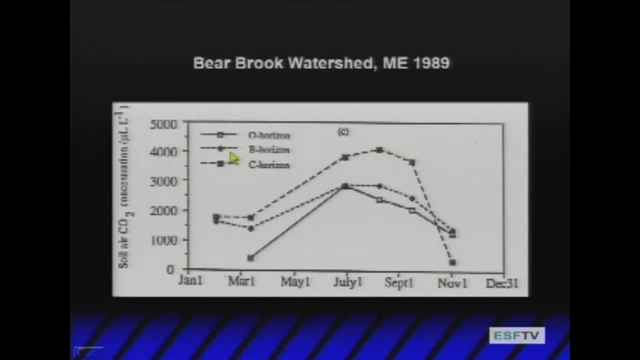 what is that in percent and how does that compare to an ag system? So again, I'm going to leave that to you and I'm going to ask you to convert that And when I see you again in person I'll ask you for those numbers. 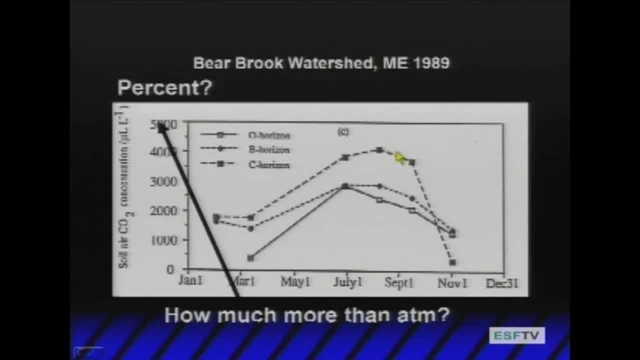 And that begs the next question: In this system, how much more is this in the soil relative to what's in the air? What's the factor of increase? So three questions for you to answer when I see you next time. Okay, We've talked about it. 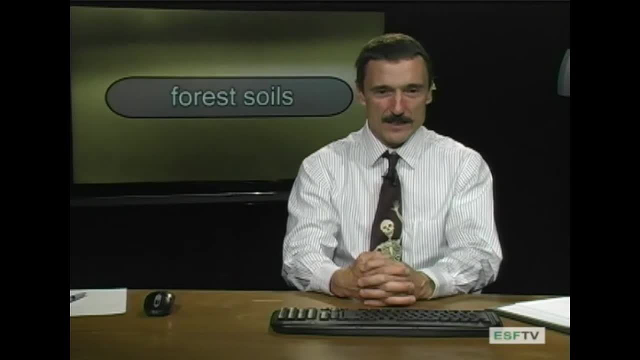 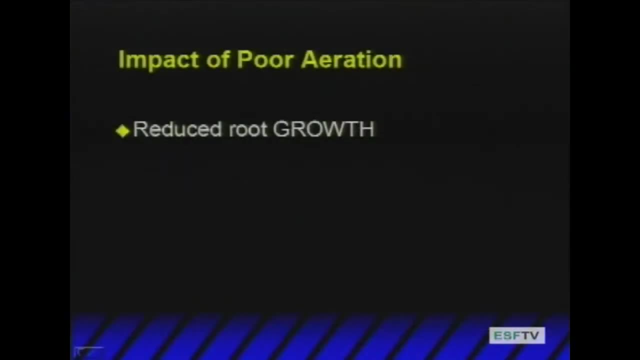 We've quantified it, We've looked at ag systems. What are the impacts of poor aeration? Well, the first and obvious one: reduced root growth. And we think back to that graph with the oxygen diffusion rate and that, 0.2 times 10 to the minus 6. 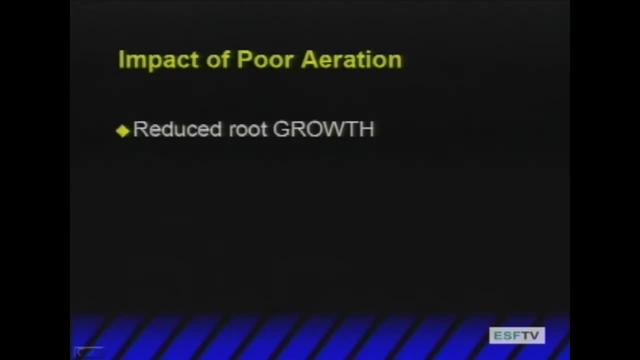 microgram, or centimeters squared per second. That's clearly reduced root growth, and when you have those high concentrations, the roots cannot respire and they stop growing and sometimes they can even be killed. So it's not only growth, but roots have a function. 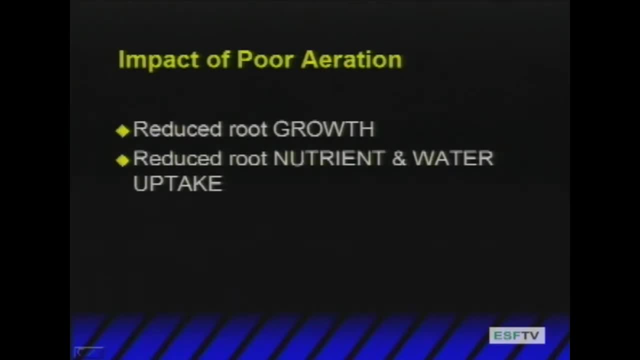 and their primary function, aside from stability, is to uptake nutrients and water. So as the CO2 concentration increases, the O2 decreases. as aeration becomes more poor, root nutrient water uptake ceases. So that's a direct result. Now these are related. 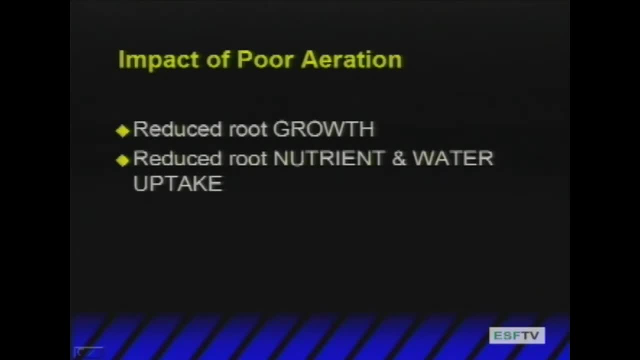 because that of course impacts growth. The microbial decomposition rates slow down. Last week we visited organic soils and those organic soils were there because the rates of accumulation far exceeded the rates of decomposition. And those are in wetlands, Of course. in wetlands the reduced oxygen levels 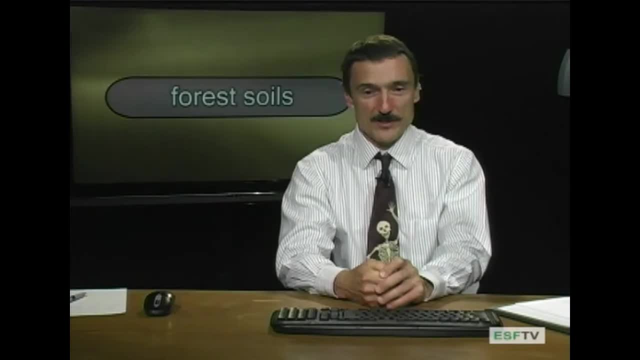 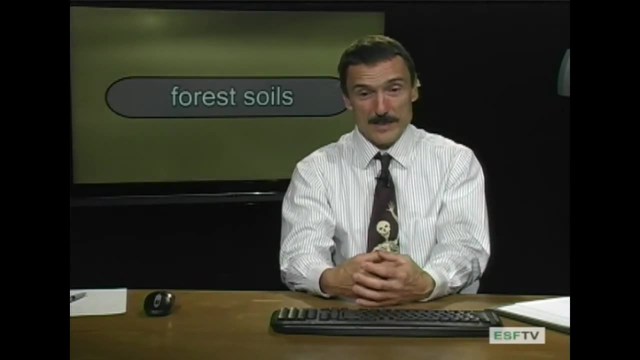 are very, very low, practically nil. There are anaerobic conditions, so material doesn't decompose, it builds up. That is a negative impact. This microbial decomposition rate in upland systems is pretty important because it's responsible for cycling of nutrients. 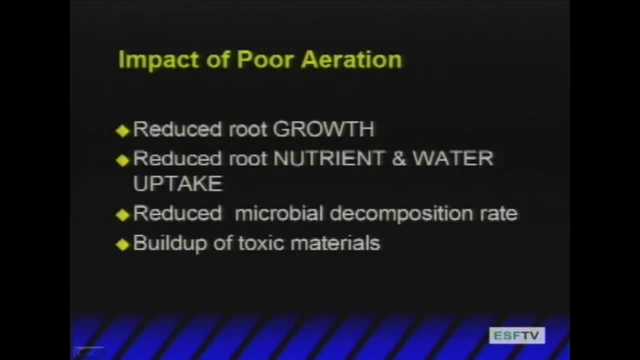 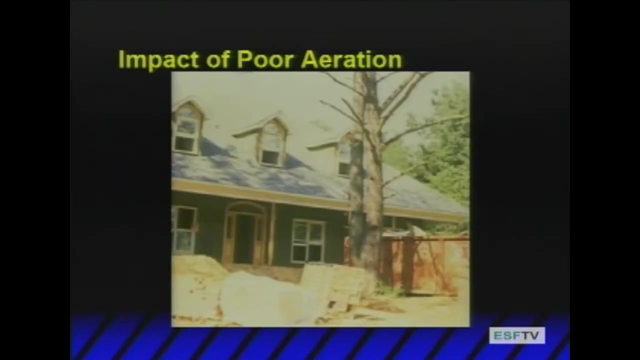 Another consequence is build up of toxic materials. Some of these gases- methane, hydrogen, sulfide- these are toxic. CO2 is toxic and those materials build up and they contribute to the inability of roots and other organisms to function. Here's a nice slide. 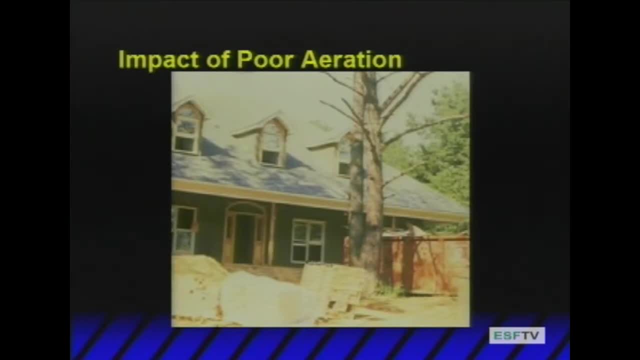 depicting active negative impacts on perioration. Many times you see this in a development: So here's a tree, the homeowner desires a tree, brand new house and all around the street there's no protection to the soil. So immediate first thing is soil compaction. 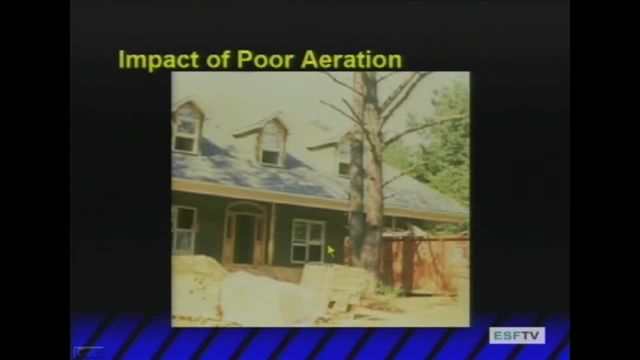 and increasing in the density, But the associated problem with that is the decrease in macropore space and a subsequent decrease in aeration, And this is often the death knell for the tree. There are a whole lot of species that just cannot handle this. 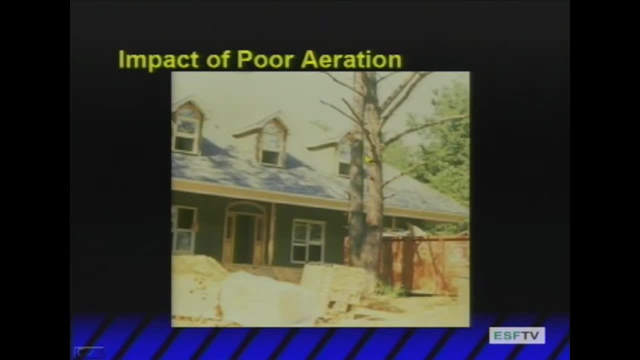 So, two or three years after, the developer made a $5,000 bill to remove this tree between power lines, and it costs anywhere from $1,000 to $5,000 to have this done, depending on the tree size And if you don't take care of it. 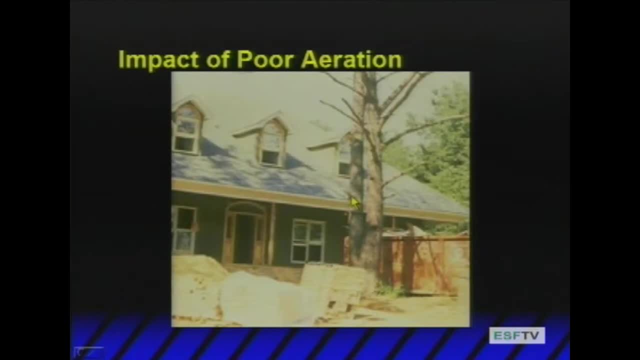 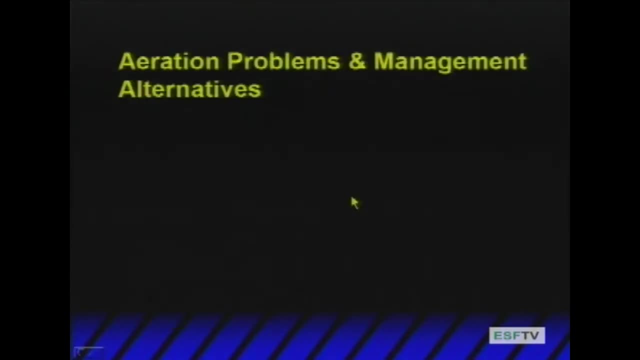 of course, the next thing you have is a lawsuit when it falls on someone else or someone else's house. So what are some management alternatives? What can we do when we have poor aeration? What are some solutions to this possible potential growth limitation? 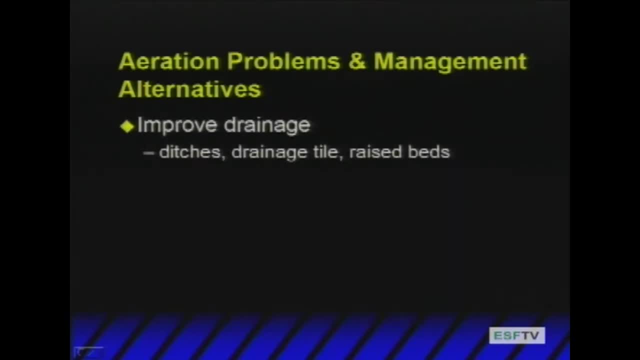 Well improved drainage And we talked about this. We call our soil water lab. We talked about the effects of ditches and drainage tiles and raising beds. By doing that you can get the aerated zone thickened or increase the aerated zone. 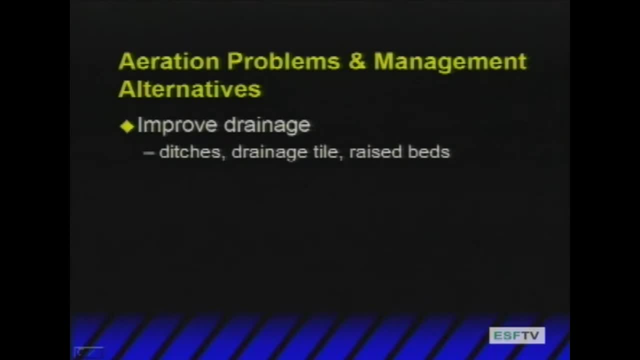 And we showed how to space drainage ditches- and we talked about this in drainage tiles and we actually looked at this in our organic soils lab. We saw the various drainage tiles and ditches and saw how low the water tables were. So that's one way to do it. 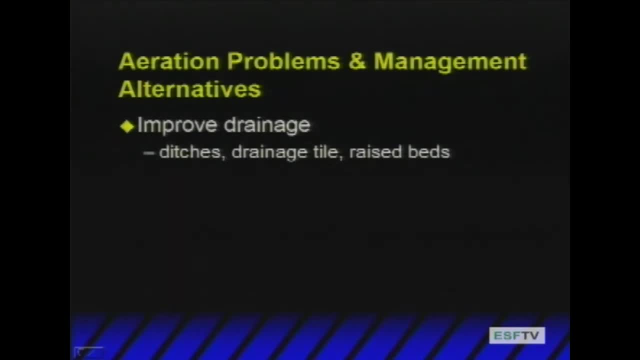 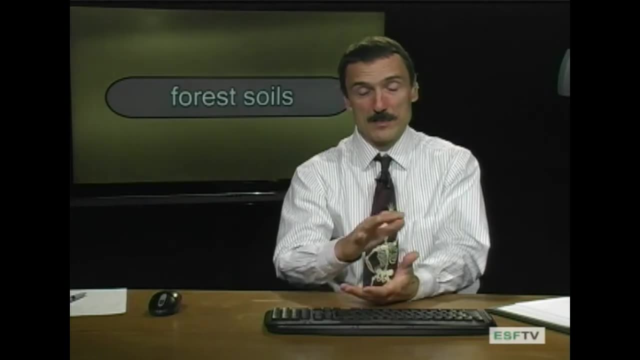 It may be practical on large areas. If you're growing vegetables, it's practical. It used to be a very practical way to increase the growth of southern pines in the coastal areas. A system of drainage ditches made a tremendous difference in the growth of pine. 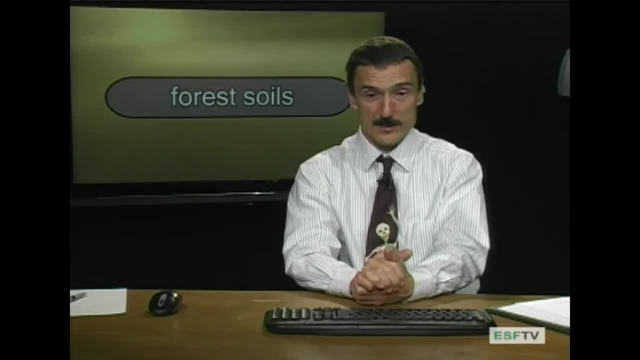 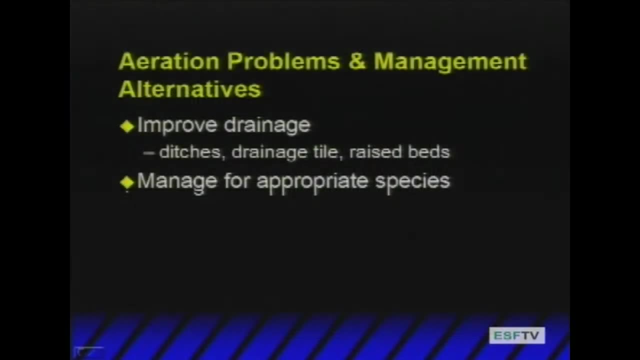 from non-commercial to commercial. So a lot of drainage ditches were installed in the southeast in the 60s and 70s. Another way to do it is to just accept poor drainage or poor aeration and utilize the appropriate species. There are a number of species. 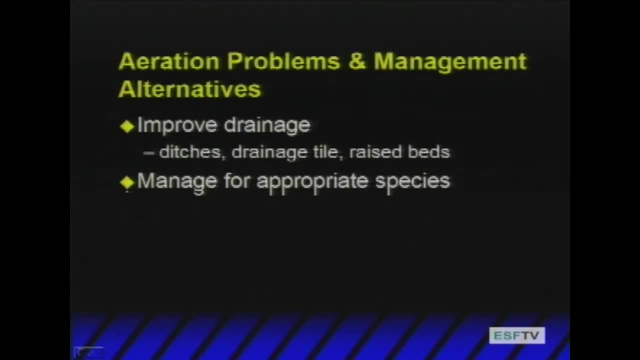 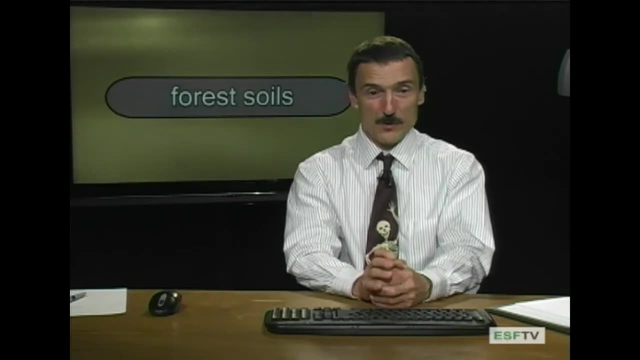 that are able to effectively compete in poor aeration: Black spruce, for example, and we've talked about some of these in the past. Red maple can handle some pretty wet conditions. What are the species that can't? And think about our trip. 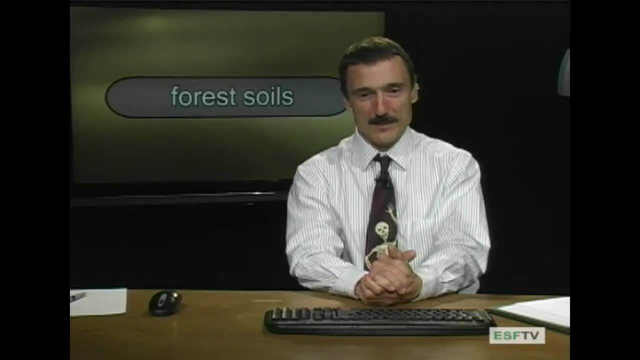 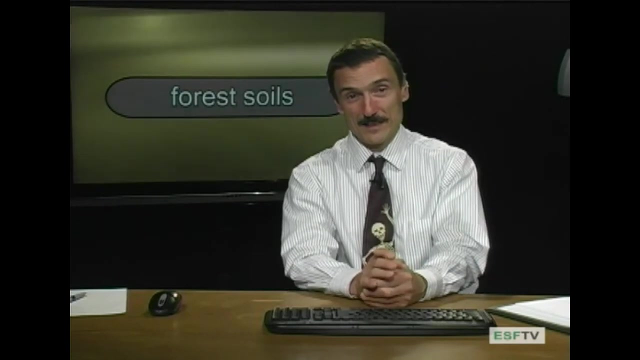 to Three Rivers, our first field lab in terms of soil morphology and the red pine, And they were doing extremely well in that very well-drained- somewhat excessively drained- Otisville soil. Then next week we visited Hivert Forest And we looked at red pine. 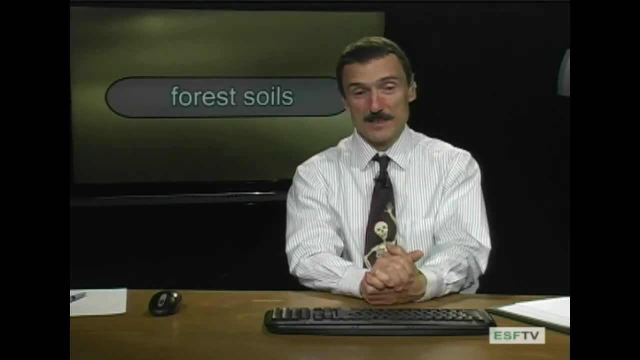 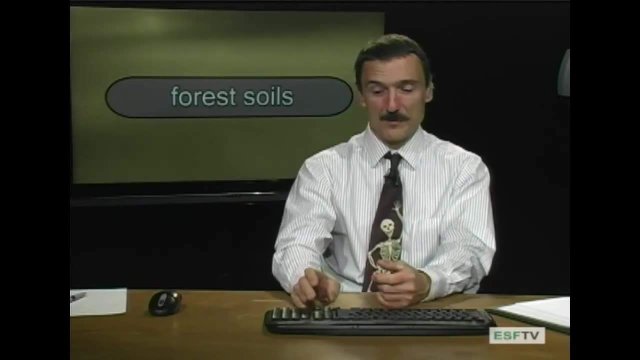 And essentially it was dead pine. So just simply managing the correct species is a very important piece of this, And that's one thing that ties the utilization of soil information to land management And large land pieces. it's really often not available and resources aren't available. 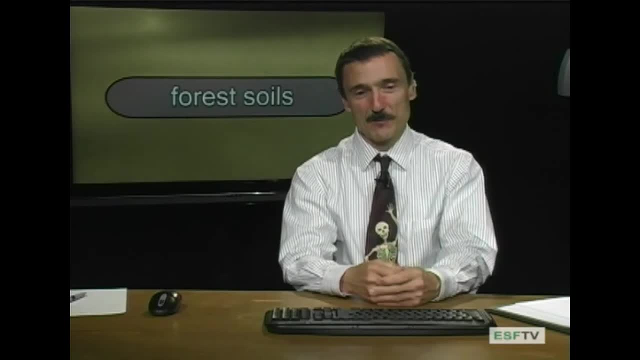 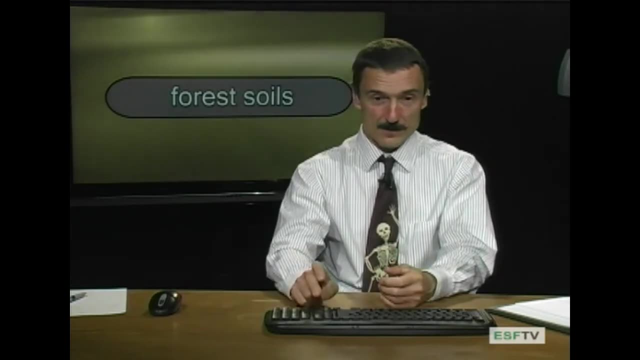 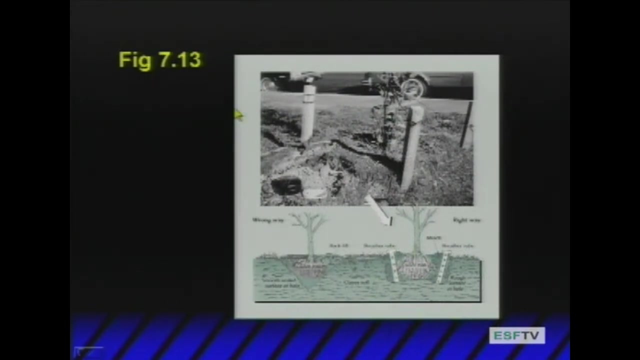 to be able to do these massive changes of aeration. And so then we're kind of dealt the hand and you've got to manage the hand you're dealt with And that's by managing the appropriate species. Another way to improve aeration is with aeration tubes. 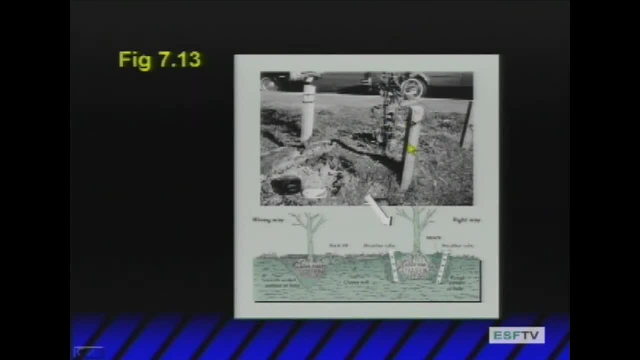 So a lot of times in the horticulture industry you see these tubes with holes sticking out, So these are inserted in soil to actually improve root aeration. And of course in the horticulture industry there's a whole other set of resources available. 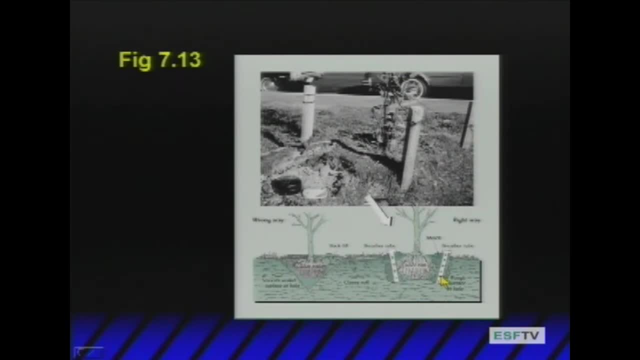 These trees, individual trees and individual plantings worth thousands of dollars in landscape context, And so the ability to treat or to manage the situation or to manage the site is greater than you have in a forest situation. There's a lot more at stake and there's a lot more capital available. 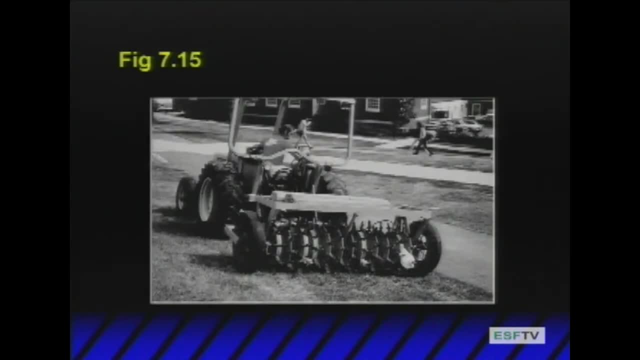 to improve the situation In lawns. there's a whole operation- ChemLawn and other companies- that make their living in making lawns lush and green, And one of those involves soil aeration. Here's a treatment that actually takes little plugs of soil out. 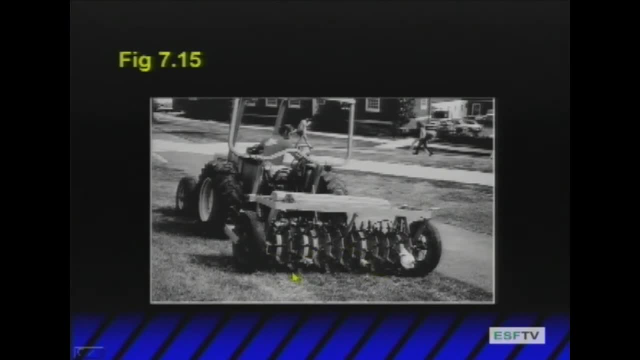 Now, it doesn't compress the soil, It takes little plugs out and provides little holes. So you see this a lot on golf courses. These almost like little tiny divots, and these holes allow proper aeration to some of these lawns. So it's not all bad. 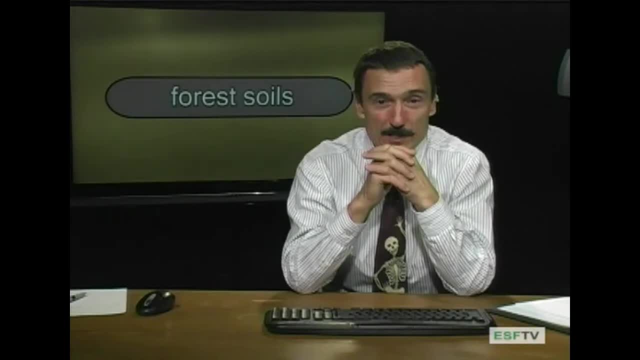 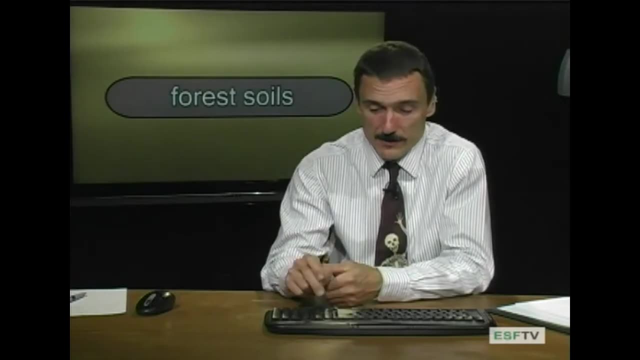 There are some very positive impacts of poor aeration, and we actually utilize poor aeration systems and we visited some of these systems. last week, We visited wetlands. We utilized the advantages of poor aeration And one of those is wetlands. And so what is a wetland? 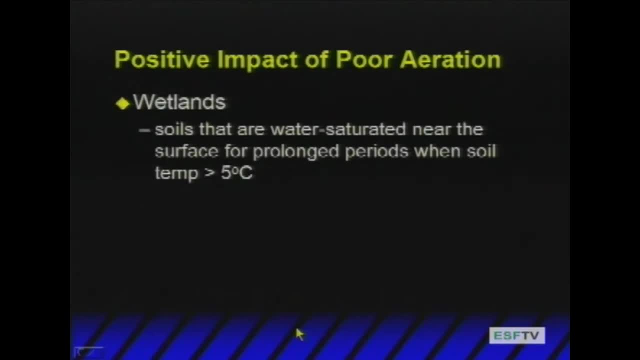 So we define a wetland as soils that are water saturated near the surface for prolonged periods. And there's a key thing here, This little piece: temperature greater than 5 degrees C. This is a key component: Saturation, before you get to the growing season. 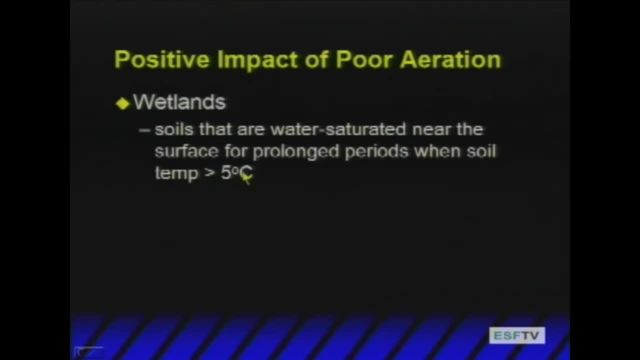 doesn't make any difference. But once you have organisms trying to subsist, once you get to this temperature greater than 5 degrees C, then it becomes important for aeration for a lot of these organisms. So the wetland definition: water saturated near the surface. 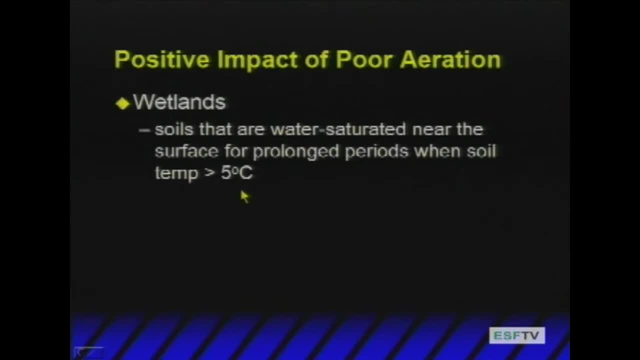 prolonged periods in a temperature. It's kind of a fuzzy definition And so that's led to a lot of problems and a lot of refinement with what wetlands are. So what are wetland characteristics? So we have to first define a wetland. 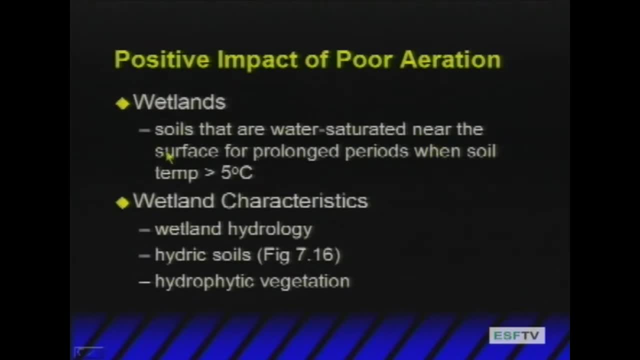 So we need a little. this is a little bit of a fuzzy definition. So we say: well, we need a little more than that to really tell what a wetland is. And so we define wetlands based on three criteria: The hydrology, the saturation. 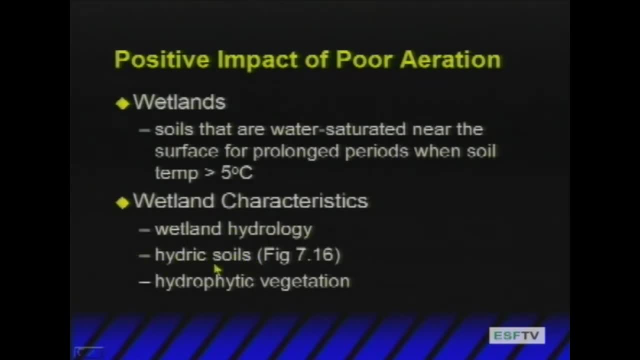 hydric soils, the presence of very wet soils, poorly drained soils and hydrophytic vegetation. So the Army Corps of Engineers utilizes these three criteria to define a wetland. And this is the beginning. These are the criteria and there are several conditions. 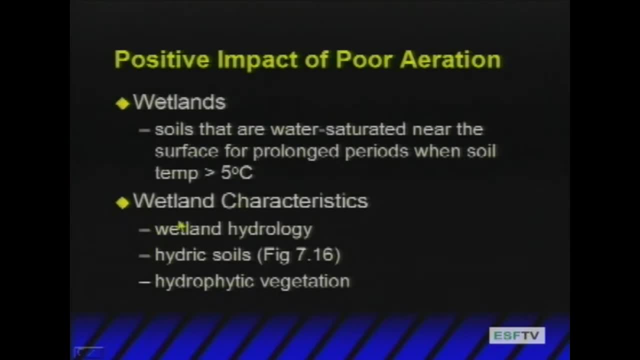 to meet each of these. So when two of these three are present- the Corps, the Army Corps that regulates and is in control of the Clean Water Act, you have a wetland, And so many of you when you get out of here in the next couple of years at a consulting firm. 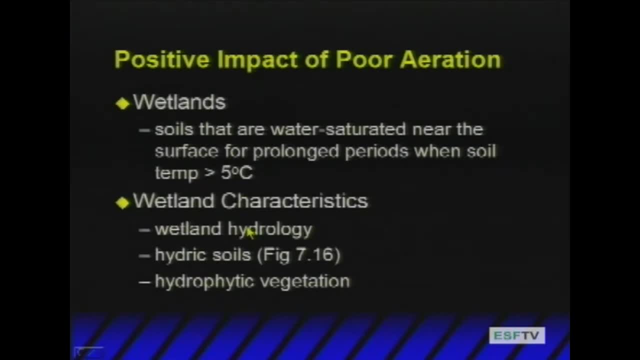 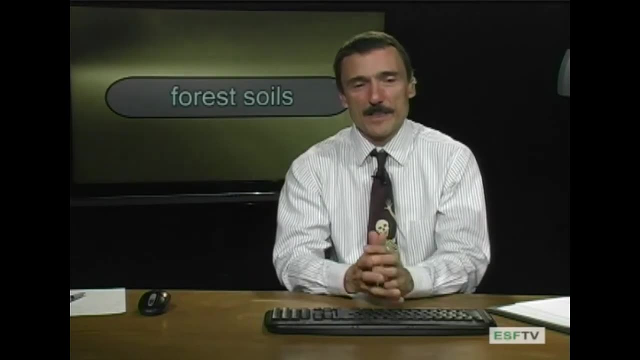 an environmental consulting firm actually might be doing some of these wetland determinations, wetland delineations. So let's look at the pieces of those. Let's first look at hydric soils. Hydric soil- So again we start with a definition. 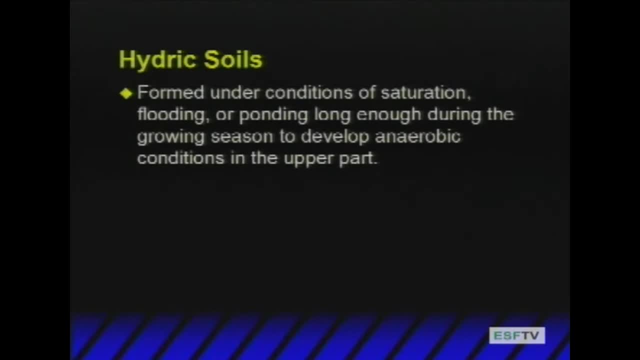 and a definition that maybe is a little bit loose and fuzzy and because of that has some indicators. But let's look at the definition of hydric soil. Hydric soils are formed under conditions of saturation, flooding or ponding, So they're wet. 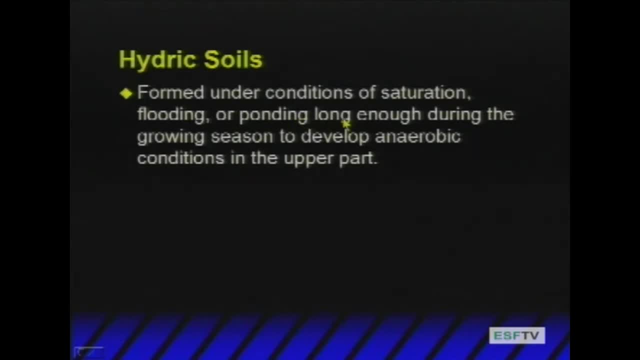 Saturation, flooding or ponding, And then, when Long enough, during the growing season, We come back to the same idea: the growing season, Temperature greater than 5 degrees C, soil temperature And long enough, and the result: anaerobic conditions in the upper part. 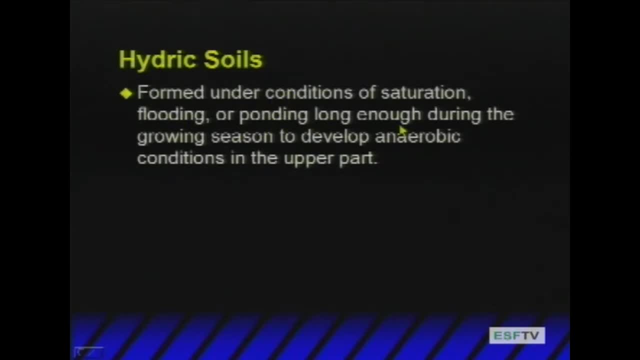 So conditions of saturation, flooding or ponding, Long enough to develop anaerobic conditions in the upper part And you might say: well, what's this upper part And how? anaerobic And long enough. So this leads to some questions. 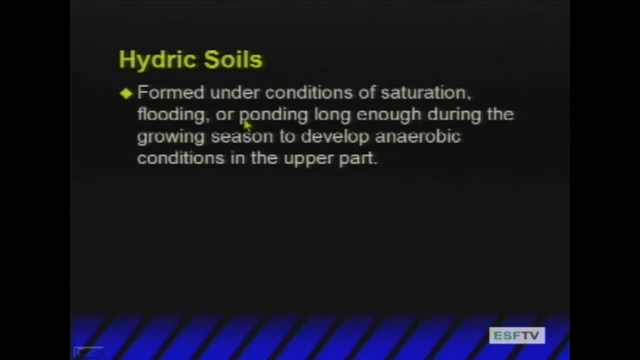 And if you were a lawyer you'd have somebody up the stand sweating. But we can solve that with some indicators, And so we go on. So saturated soils: These are saturated and reduced. A little more definitions, A little more compelling: Saturated and reduced. 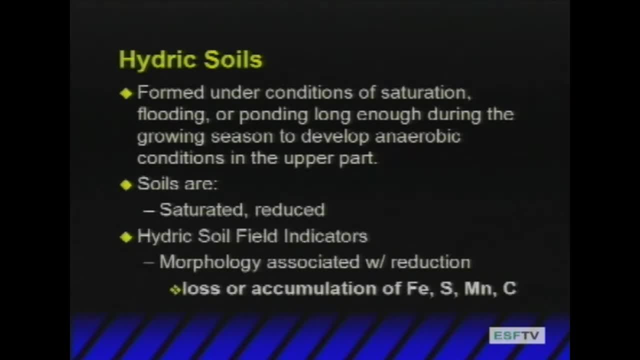 And so I still need more specifics. I'm still not very certain. I know what a hydric soil is, And so then we revert to hydric soil field indicators, And so these are indicators. these are morphological indicators associated with reduction. 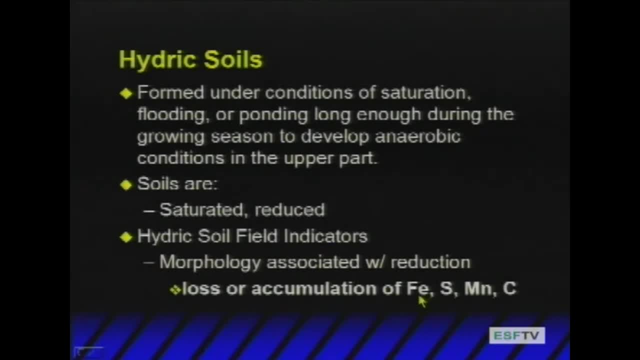 And there's lists and lists of these And here's one: Loss or accumulation of iron, sulfur, manganese and carbon. So what happens in wetland systems? Iron and sulfur and manganese and carbon- these are accumulated. Here's a depiction. 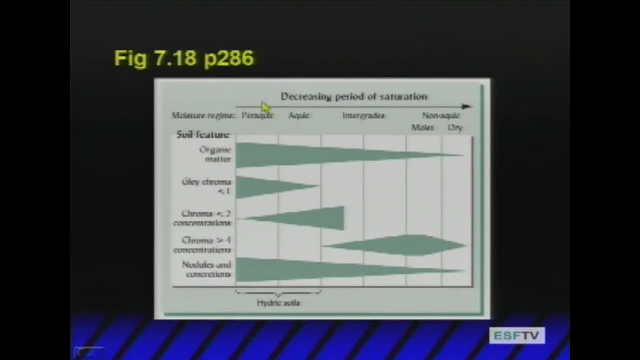 Here we show decreasing period of saturation. This comes from the text, And here we have hydric soil. So we have a couple of indicators. So organic matter, a soil feature. We have per-aquic and aqueous, These very wet moisture regimes. 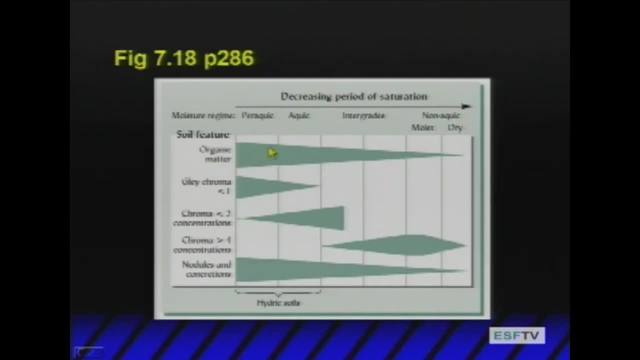 And organic matter is very high in hydric soils. And this gallea, chroma, Chroma less than one- We talked about reduced conditions- in less than two, Chroma less than two. So gallea, even grayer, less than one. 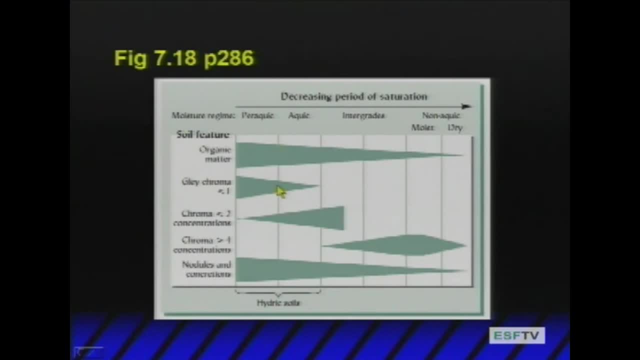 So less than one on that. remember, on the lightness chart, on the chroma chart, When you have over in those left hand columns of very low chroma, those are hydric soils Less than two in concentrations. So concentrations are small. 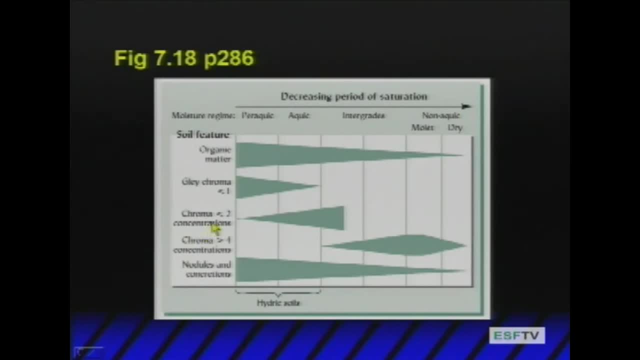 almost like little pellets, Small round, almost like pellets, And that's manganese And that gets reduced Concentrations. those are hydric soils, Chroma greater than four, Nope too bright, And the other one is concretions. nodules and concretions. 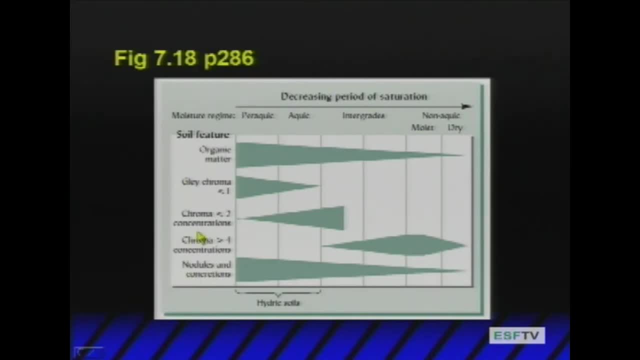 So concretions are these very hard concentrations. They're self-formed and they're manganese, And so when you have a lot of those, those are hydric soils, Those are hydric soil indicators. They help indicate the presence of a hydric soil. 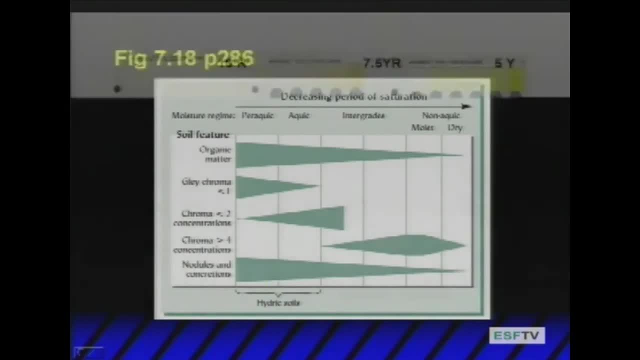 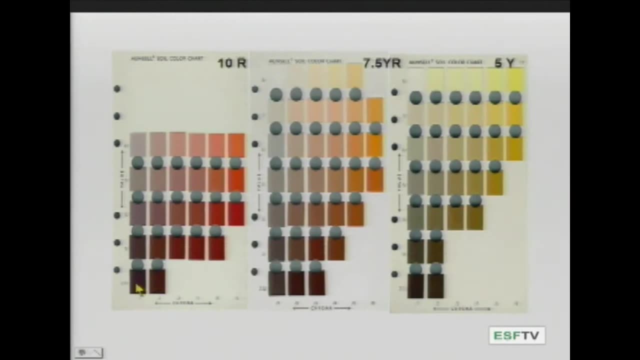 It's a little bit more fulfilling than that definition. Long enough and wet enough. Here we go back to our color chart And remember low chroma, So low chroma. we're looking on these. here's chroma one For 10R, 7,, 5YR and 5Y. 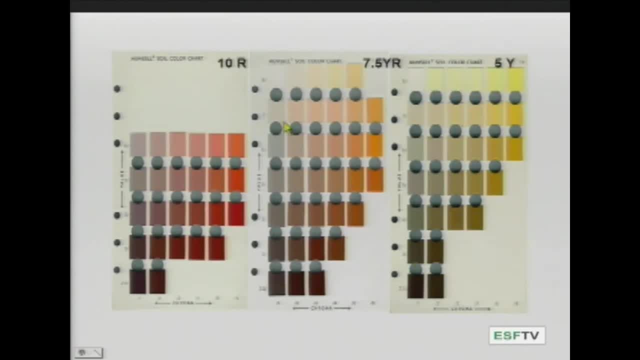 And we're looking for these low chroma, these gray colors. Here's gray with a lot of red in it. Low chroma: less than one. Those are wetland hydric soil indicators. Here's the next one Example. 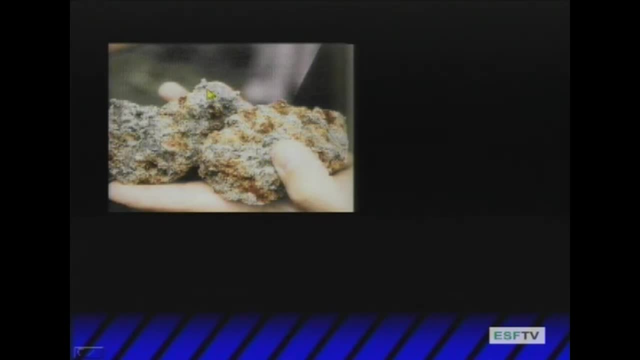 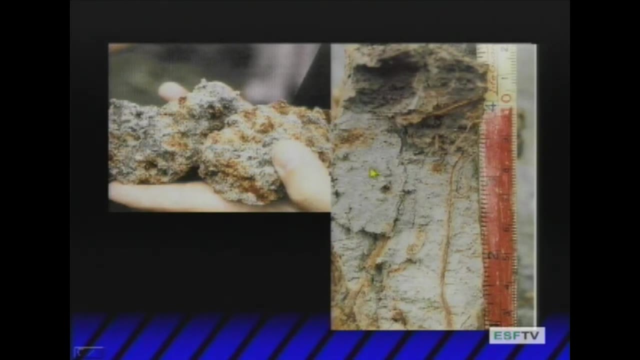 This is low chroma. This is also modeling. This is chroma two modeling. That's a hydric soil indicator. Here's very low chroma one And here are oxidized root channels. So this is another indicator of a hydric soil. 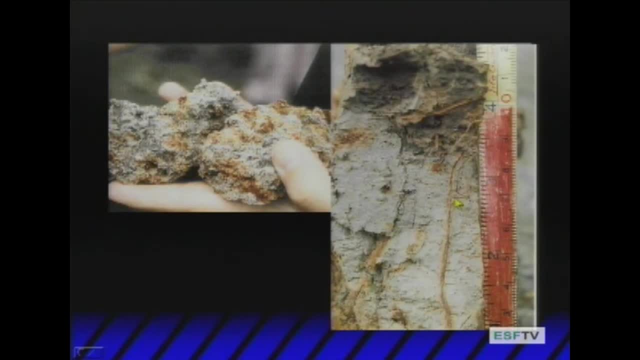 Low chroma and oxidized root channels, This root channel standing. So the root oxidizes iron just around the edge and everything else is reduced. Of course, that root's pumping iron down. here It's pumping oxygen down. Here's an illustration. 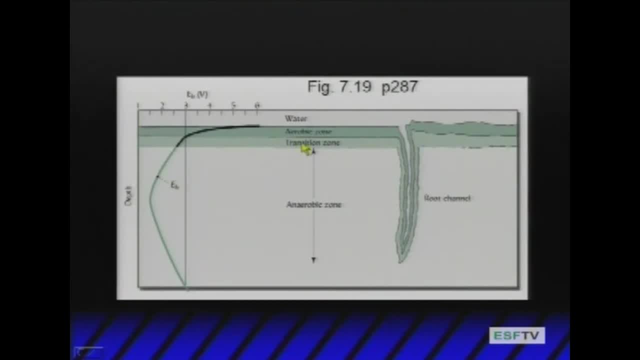 with depth and EH. So here we have water And as we get the EH decreases, You get this little aerobic zone, Transition zone. Then you get into the saturated zone. You can see the EH take a dive. So here's a nice indication of the effects of saturated 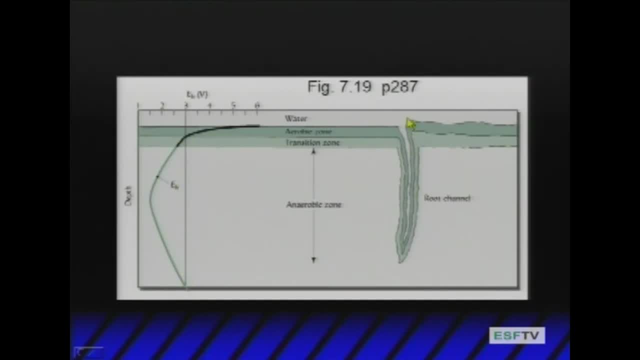 on EH, on depth And the anaerobic zone, And here's an illustration of that root channel. You can see the water comes down, But in that root channel iron is actually oxidized, So the EH is a little bit higher. 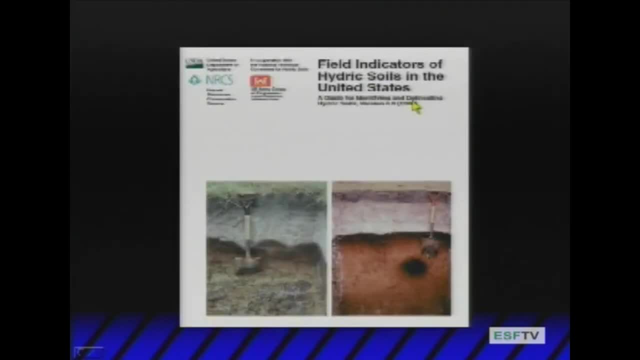 And you can look at this up. There's a nice booklet published by the USDA Field indicators of hydric soils in the United States And all these and many others are in there And this is what soil scientists use. So if you go out with the Corps of Engineers, 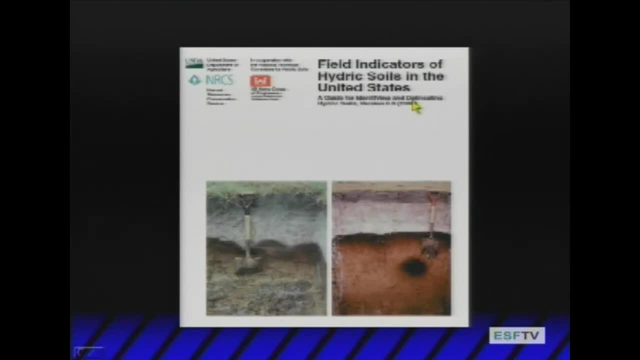 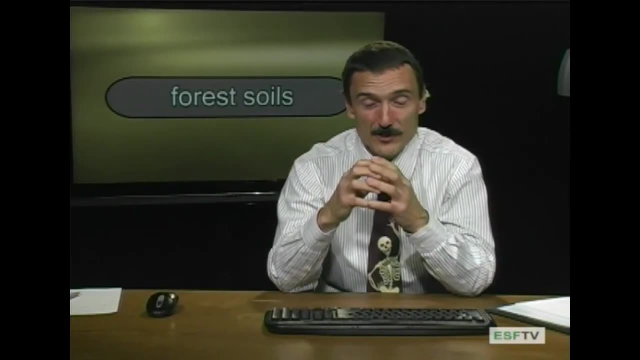 on the soil science detail. you'll be utilizing these indicators to define hydric soils which are part of this wetland. This is a person specialist doing the vegetation, Or by then you may have learned all the vegetation- The facultative anaerobes. 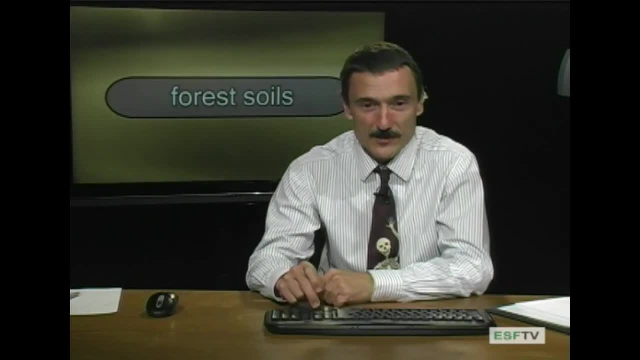 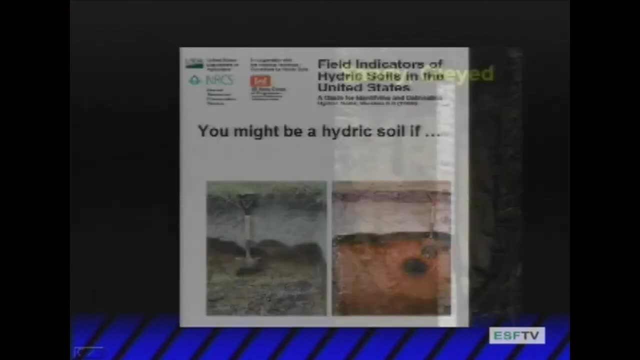 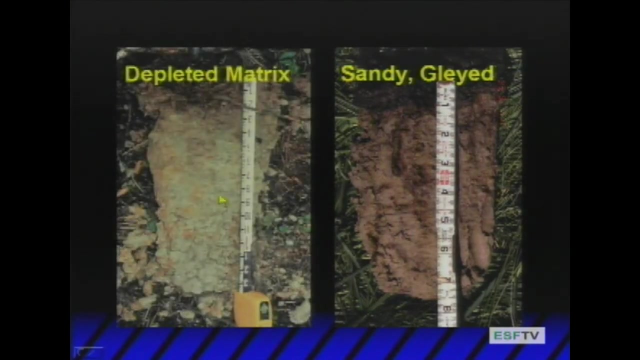 and all the other vegetation that qualify things for hydric soil And that's the redneck version. There's sandy and glade And the depleted matrix. Here's the removal of iron and depletion It's reduced iron And I guess that's a good place. 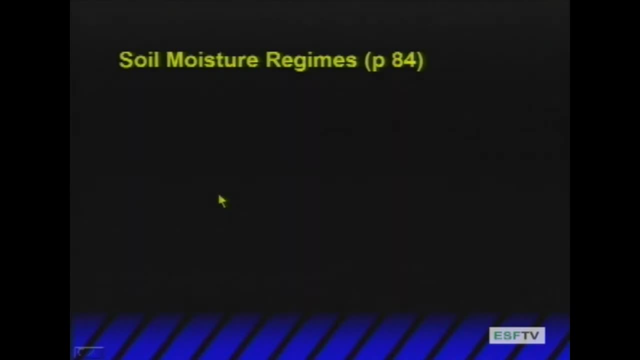 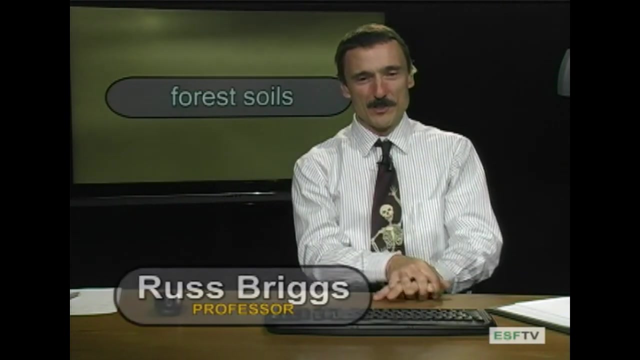 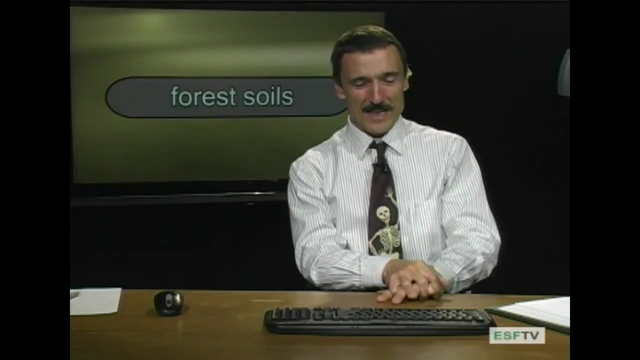 for us to stop. I hope we've digested some of this. We will continue on and when I get back we'll talk about soil temperature and we'll finish up soil moisture regimes. Hope that you enjoyed the exam and did well, And I will get those graded over this weekend. 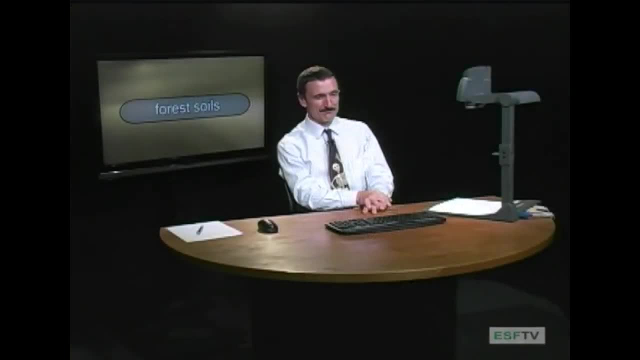 And I will see you Monday. Have a great weekend And think soil.